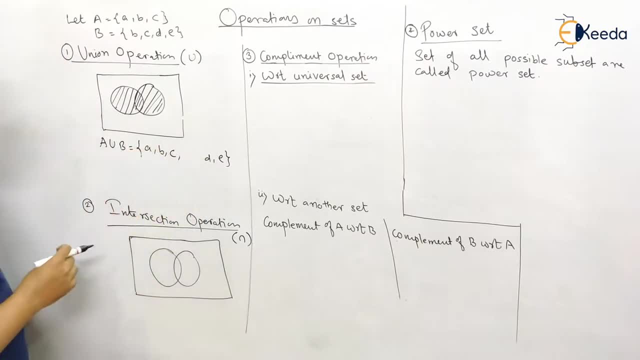 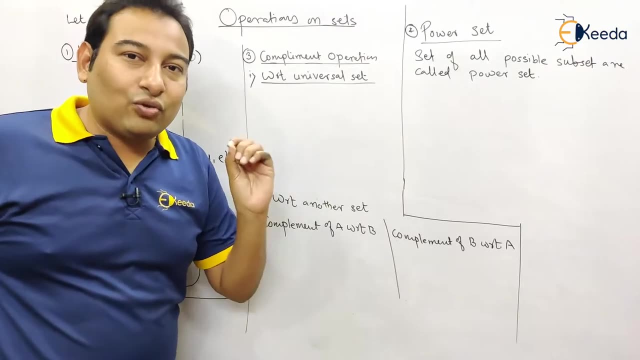 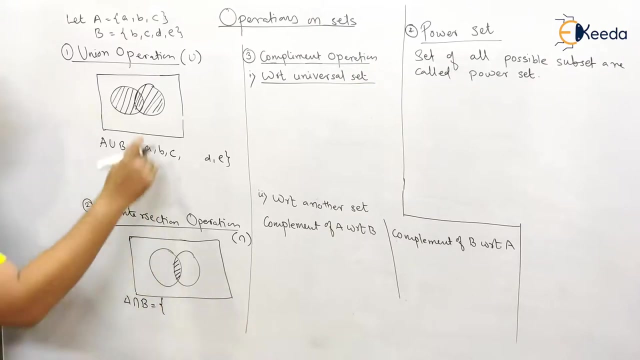 is B, C. We just consider once. So this is your required solution of A union B: All the elements of A and B common elements, we're going to consider once. So this is your union Next, intersection means common part, So what are the common element between these two sets? 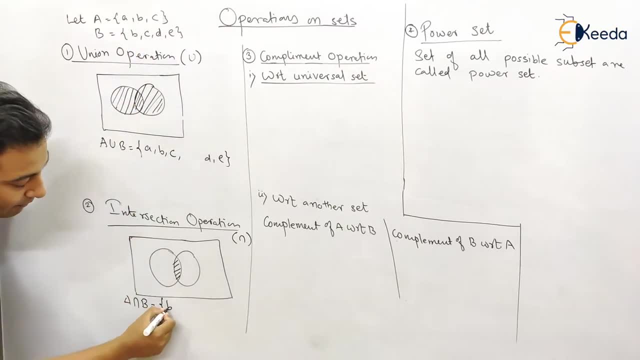 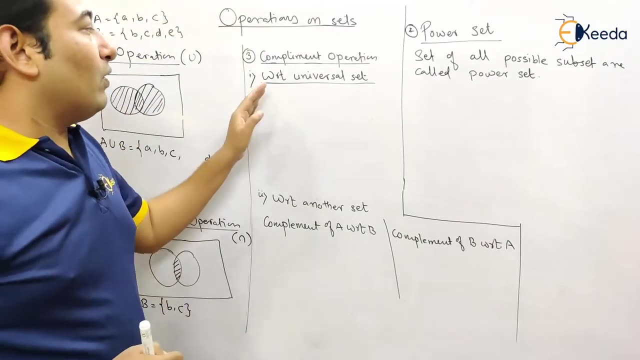 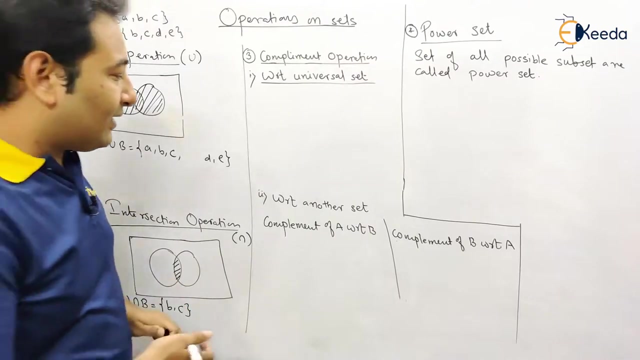 that will come under intersection. So the common is B C, So B C will come here. What is the next operation? The next operation is complement operation. Now, complement operation. there are two complement operation: The first is with respect to universal set and the next is with respect to another set. 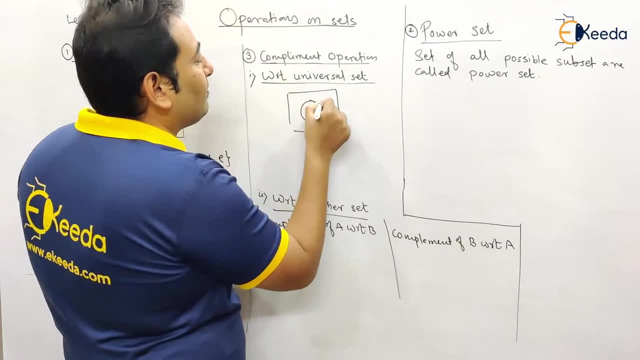 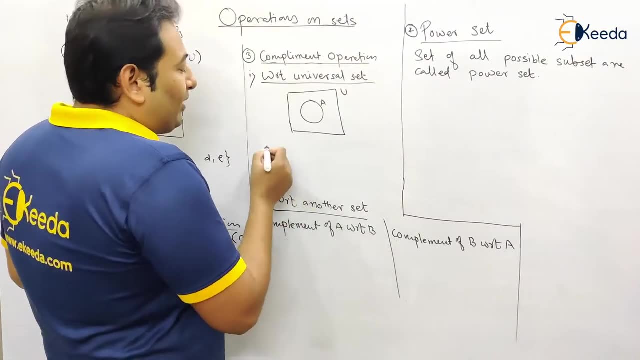 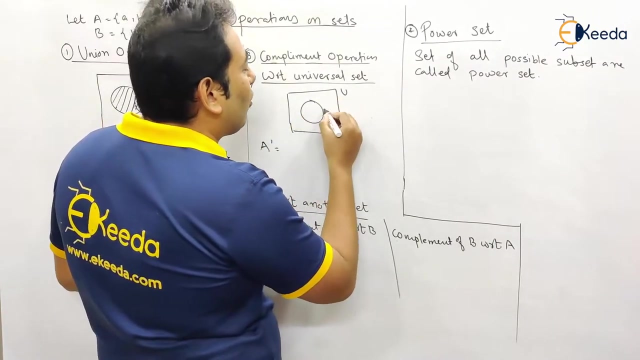 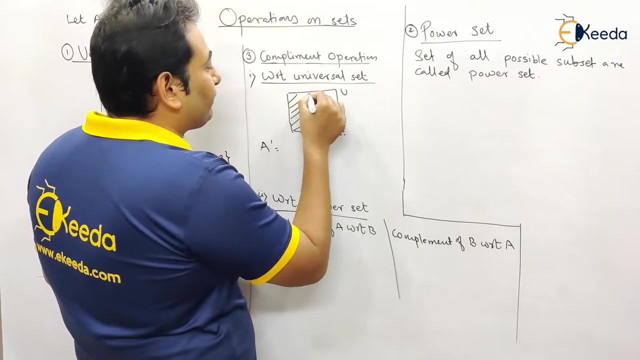 So let's discuss this. This is my set A and this is the universal set. Okay, If I'll say complement of A with A dash means complement of A with respect to universal set. So it simply means all the elements outside A and inside universal set. This is your A. So complement of A means. 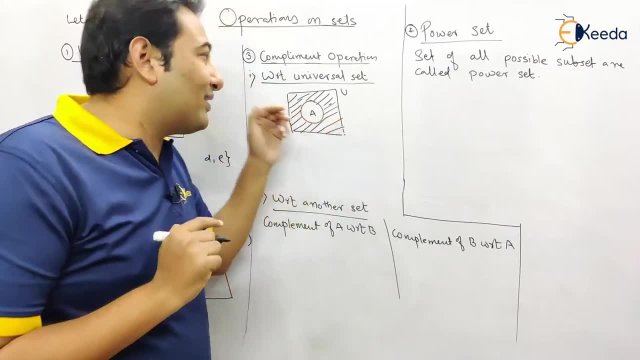 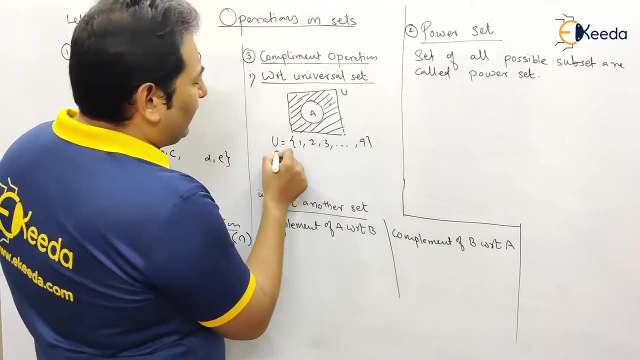 all the elements which are outside A and inside the universal set. So suppose let's say universal set is, let's say, 1,, 2,, 3, up to 9. It can be anything. And let's say A has elements. 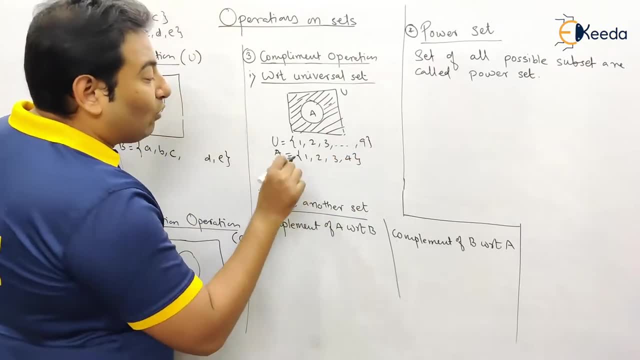 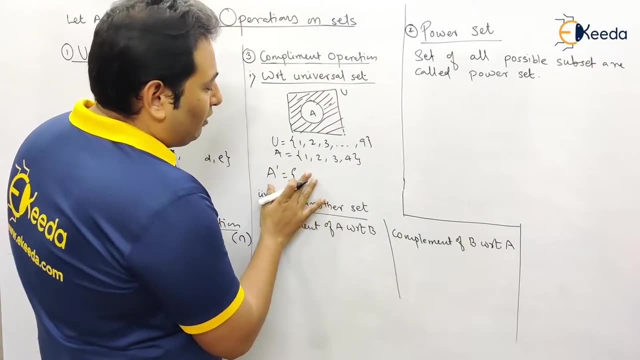 1,, 2,, 3,, 4.. Now please tell me what will be A complement outside A and inside universal-SET set. So the elements will be 5,, 6,, 7,, 8 and 9.. So this is your A complement. So, in case, 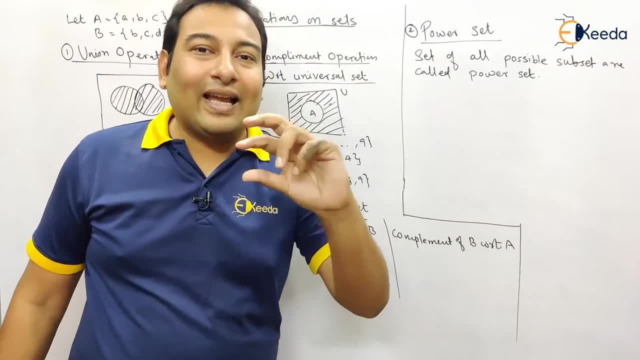 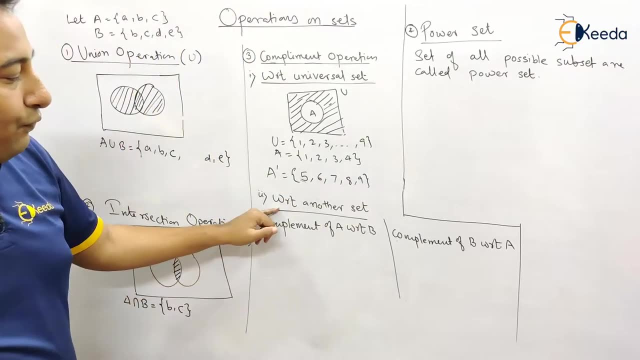 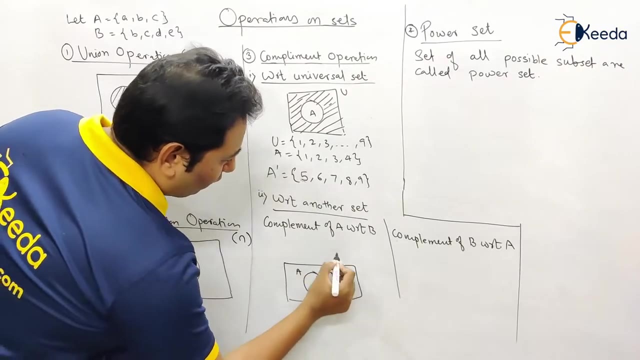 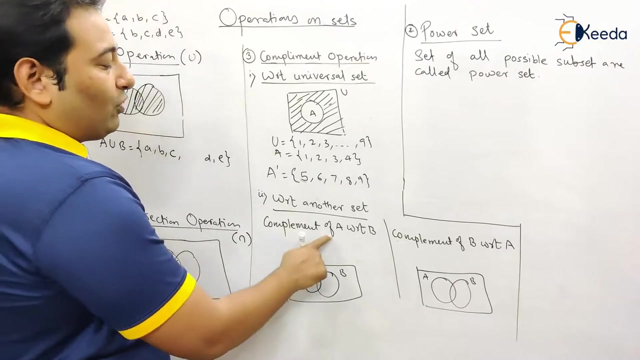 of complement. remember: whichever complement, the elements will be outside that set. Here it is A complement, so element will be outside that set. Now we'll see with respect to another set. So let's say here: complement of A with respect to B. What do you mean by that? It? 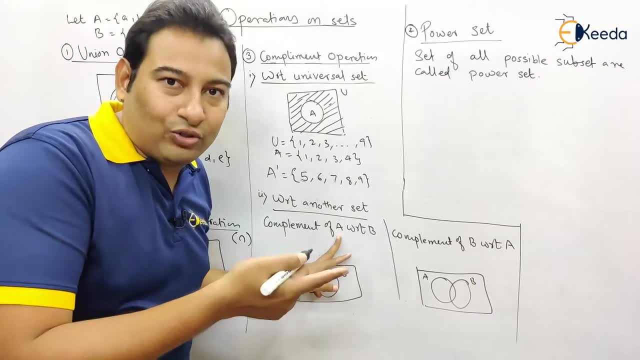 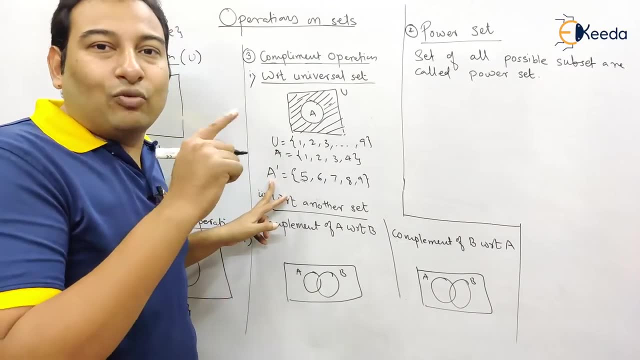 should be outside A. Complement of A means it should be outside A with respect to B, inside B. See here it was complement of A with respect to universal set. So it has to be outside A, inside U. So outside A, inside B. So please tell me which. 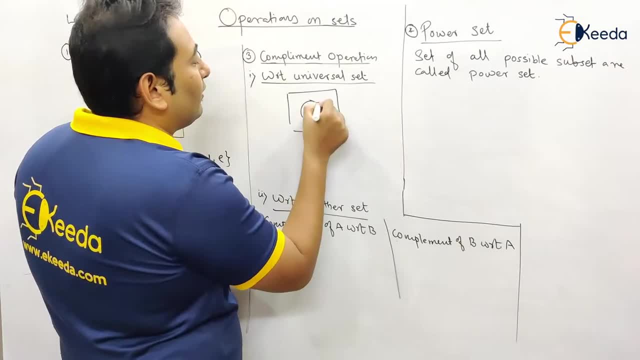 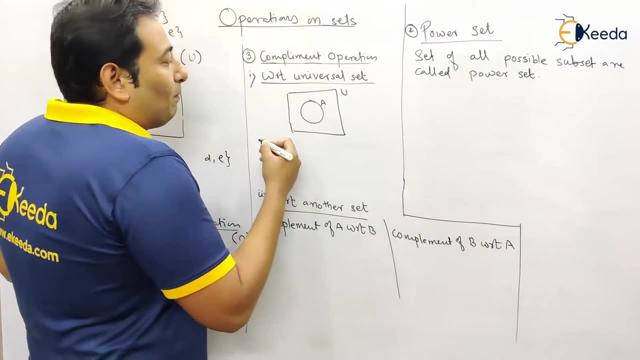 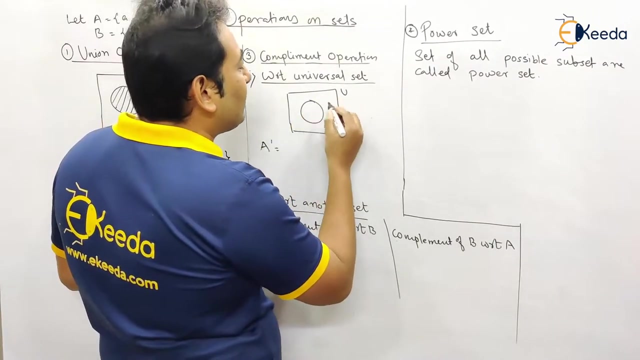 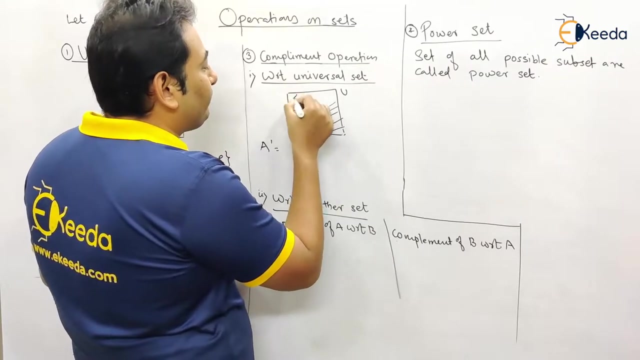 set. so let's discuss this. this is my set A and this is the universal set. okay, if I'll say complement of A with A dash means complement of A with respect to universal set. so it simply means all the elements outside A and inside universal element, universal set. 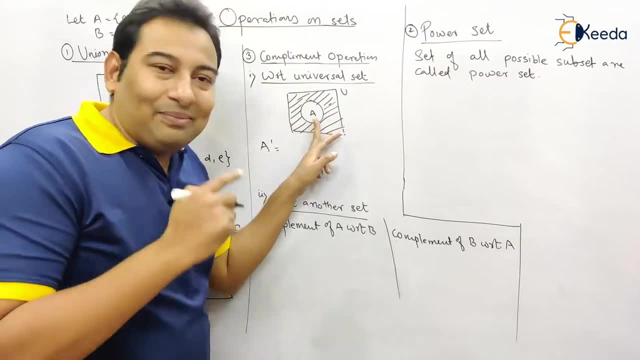 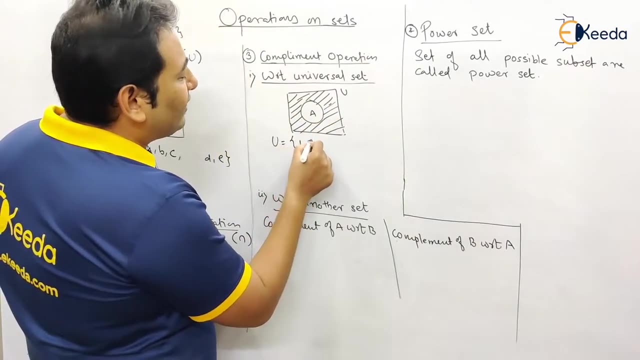 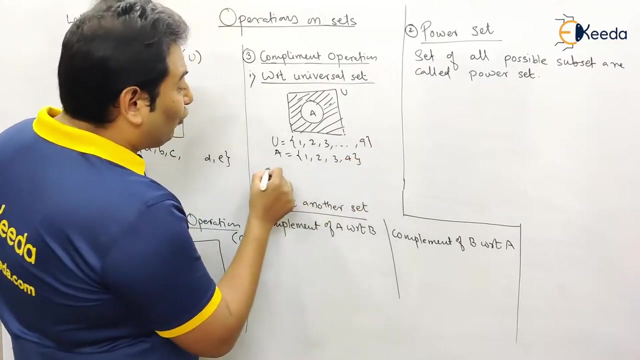 this is your A. so complement of A means all the elements which are outside A and inside the universal set. so suppose let's say universal set is, let's say, one, two, three, up to nine, it can be anything. and let's say A has elements one, two, three, four. now please tell me what. 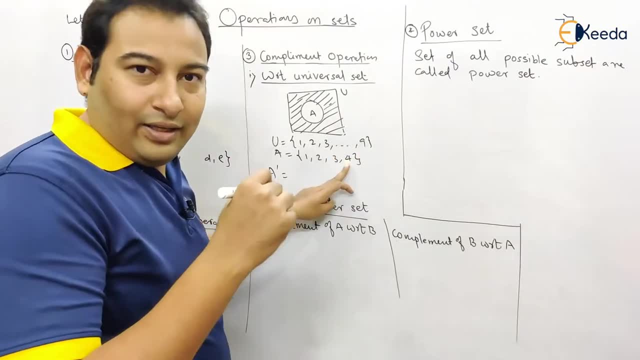 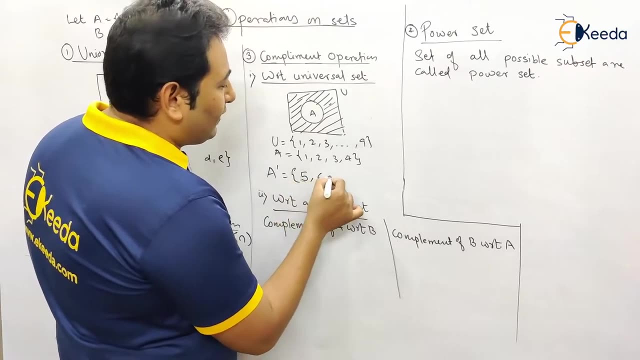 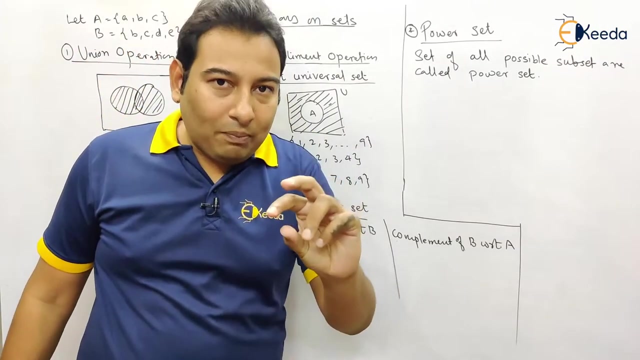 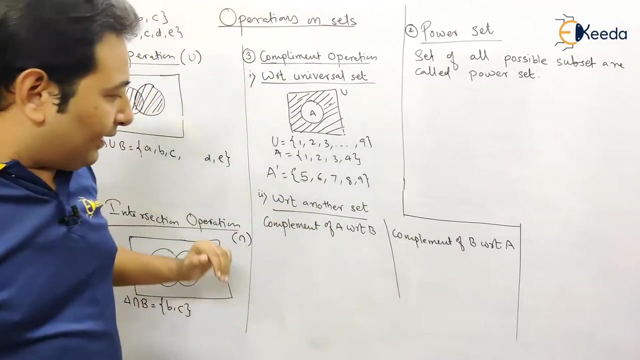 will be A complement outside A and inside A universal set. so the elements will be five, six, seven, eight and nine. so this is your a complement. so in case of complement, remember whichever complement, the elements will be outside that set. here it is a complement, so element will be outside that set. now we'll see with 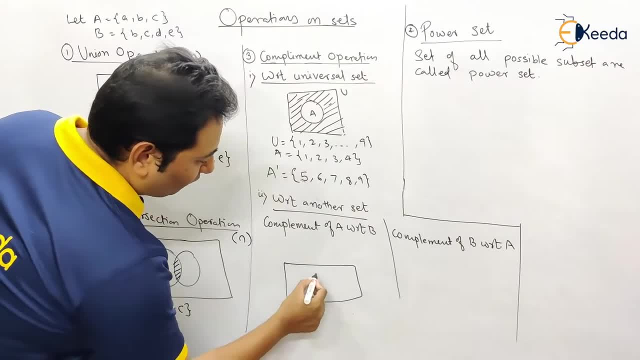 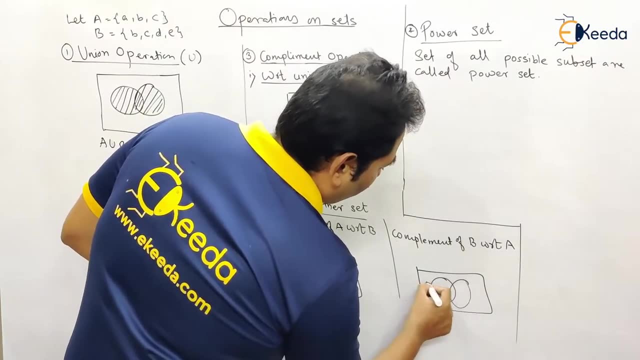 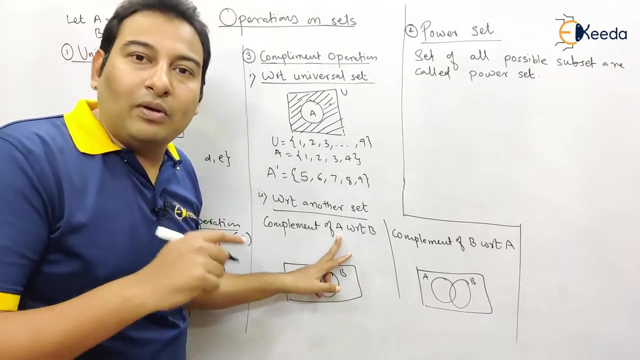 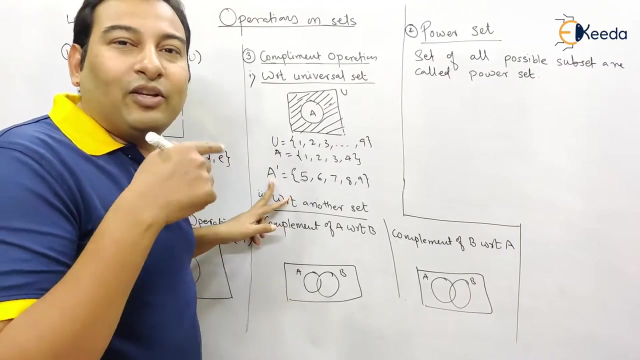 respect to another set. so let's say you here complement of a with respect to B. what do you mean by that? it should be outside a complement of him. a means it should be outside a with respect to B, inside B, see here. here it was complement of with respect to universal set, so it: 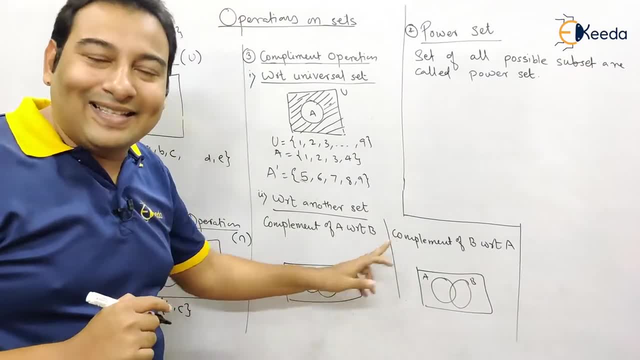 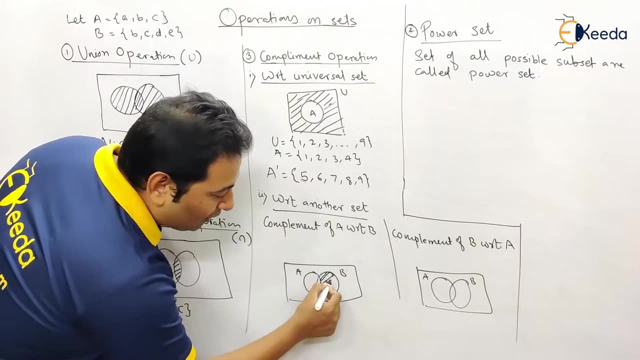 has to be outside a, inside you, so outside a, inside B. so please tell me which will be the shaded region. it should be outside a, so this is your a, outside that and inside that, so this is your a inside that and inside that, so inside B. so this is your region and it is written as B minus a. so remember the. 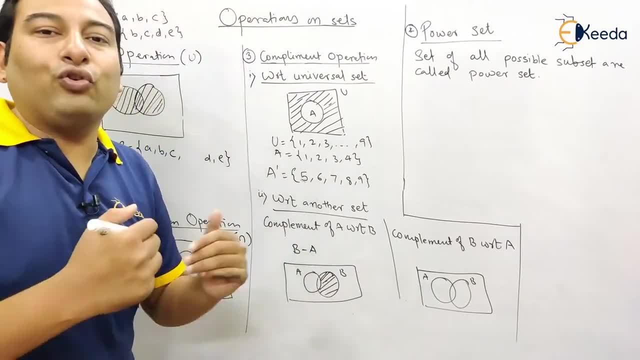 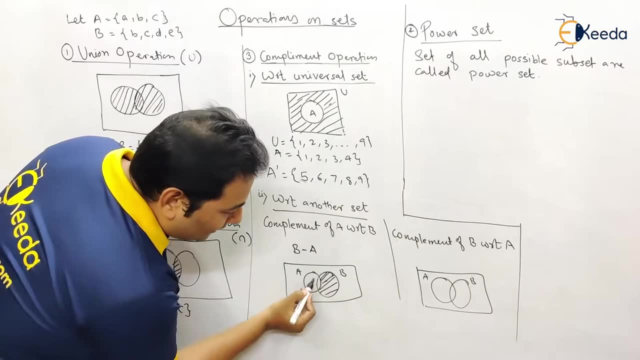 name complement of a with respect to B is actually B minus a. what do you mean by B minus a? from B: initially the entire B was selected and from this B we subtracted a- see here: from this B. if you subtract this a, you will be left with 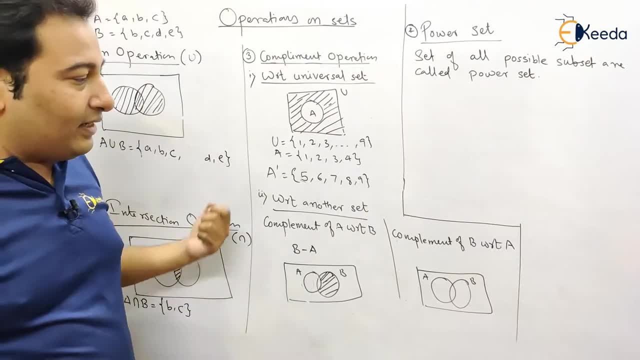 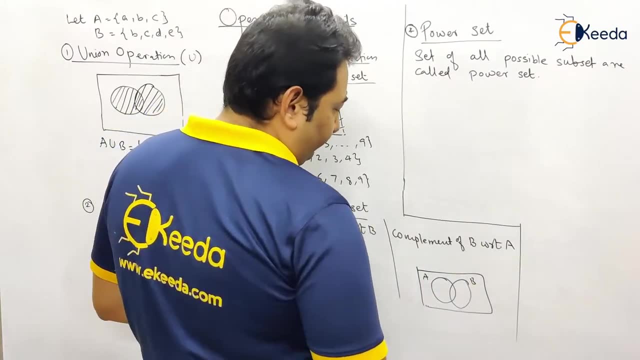 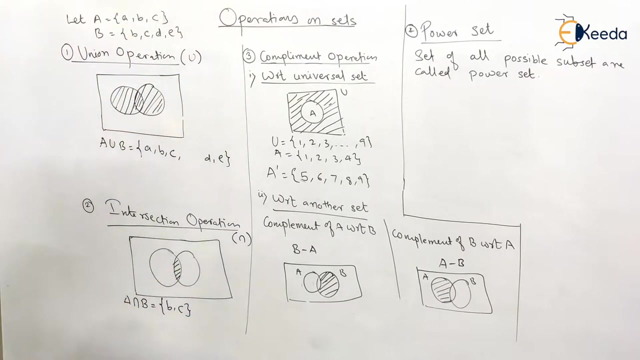 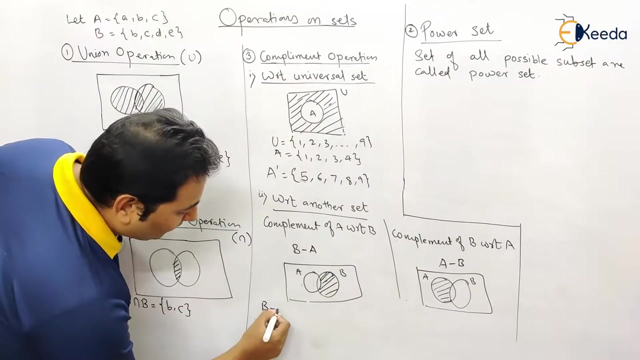 the shaded region. so actually this is B minus a and complement of B with respect to a. so that means outside B, inside B, outside B, inside. that this will be, you know, the shaded region. so outside A and this is B minus B, this is the shade of A and this will be a minus B. so if with the 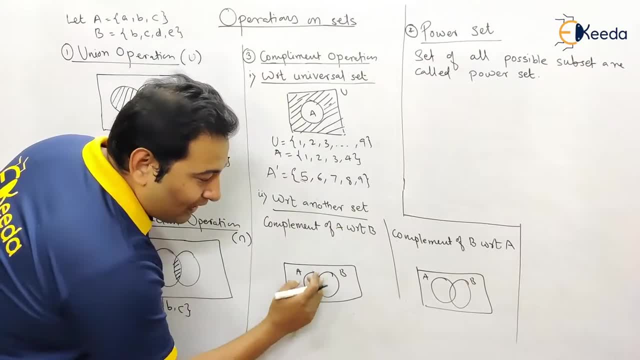 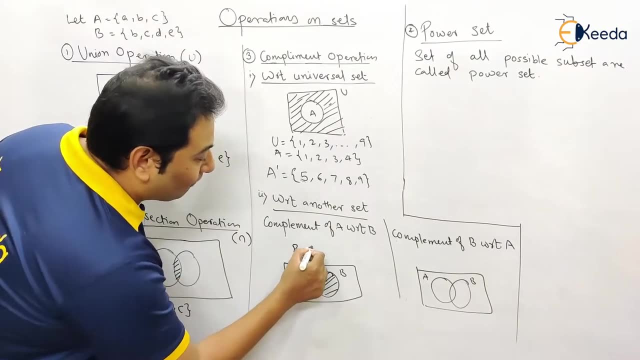 you want to see. So here it was complement of A with respect to universal set, So it will be the shaded region. It should be outside A. So this is your A, outside that and inside B. So this is your region and it is written as B minus A. So remember the name: complement. 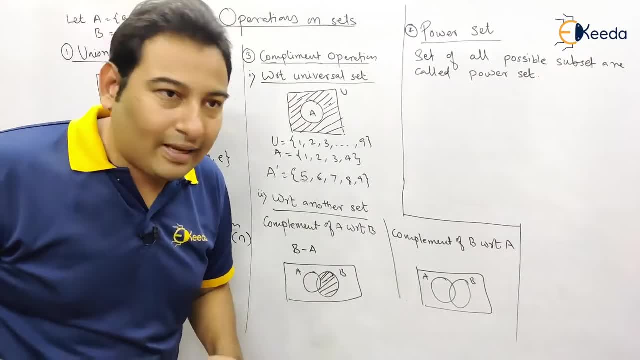 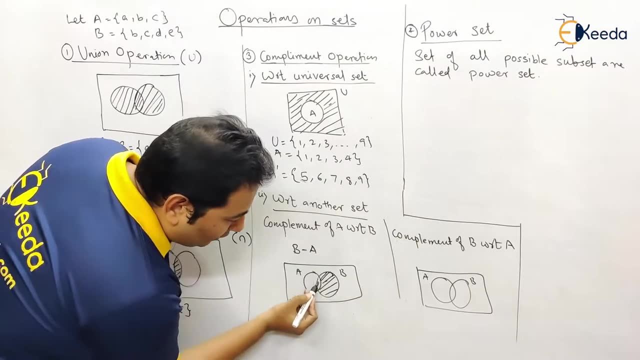 of A with respect to B is actually B minus A. What do you mean by B minus A? From B initially the entire B was selected and from this B we subtracted A- See here: from this B. if you subtract this A, you'll be left with the shaded region. So actually this is B minus A and 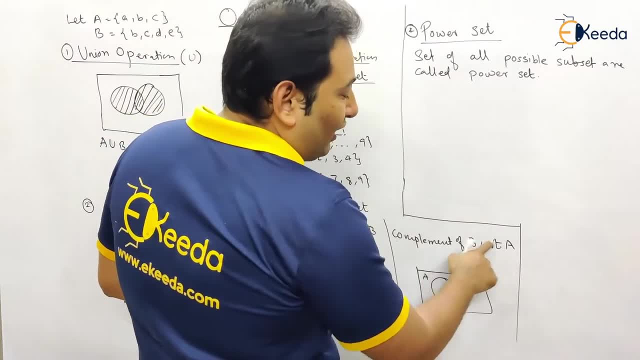 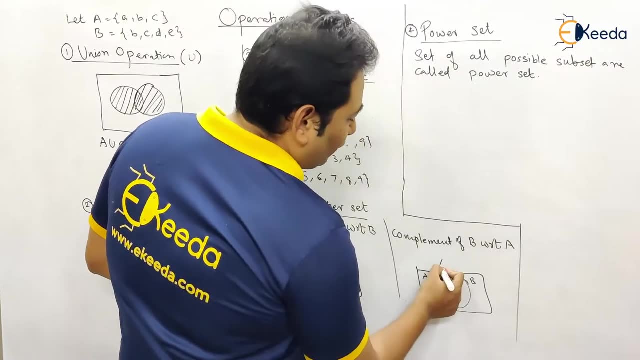 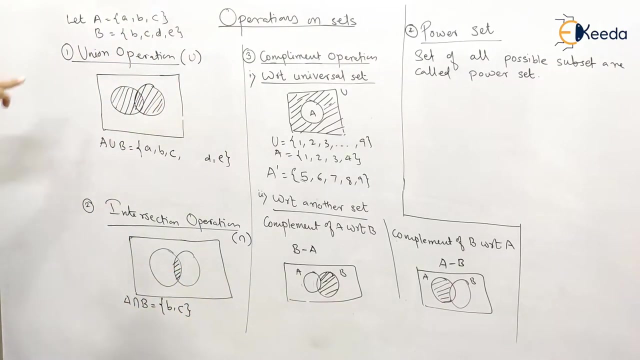 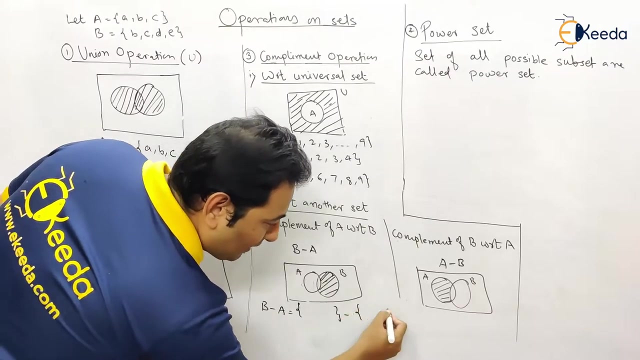 this is complement of B with respect to A. So that means outside B, inside A, And this will be A minus B. So, with the help of the same example, this example, if I write B minus A, please tell me what will be the answer. From B we're going to subtract A, Simple. 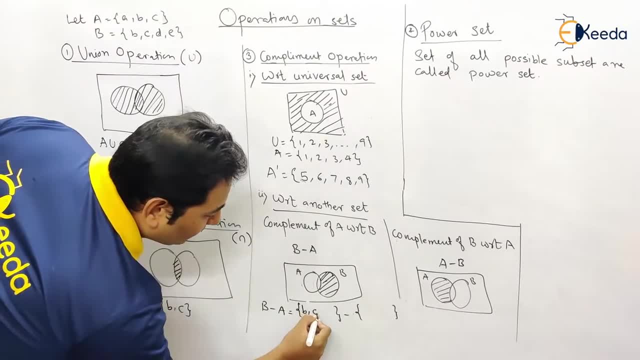 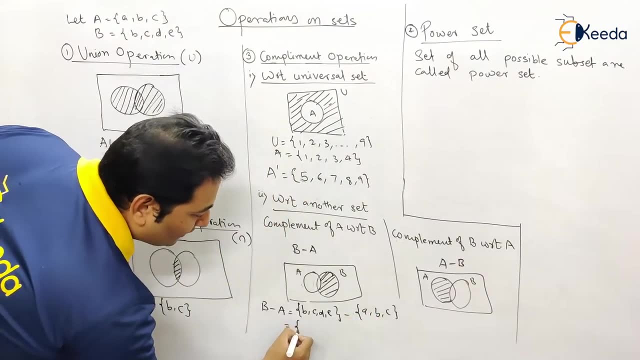 So what is B B is B C A. So what is B B is B C A. So what is B B is B C A. So what is D and E, And what is A A is A, B C. So if I subtract, what will be the result? Simply, 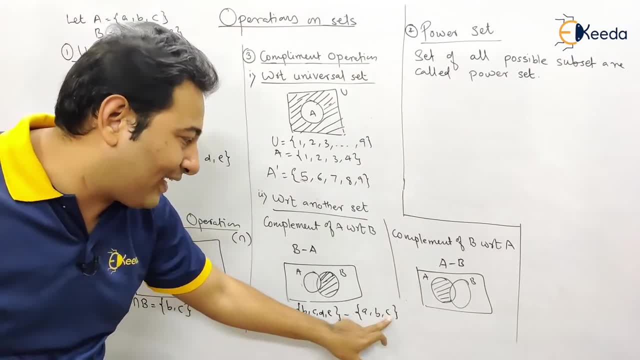 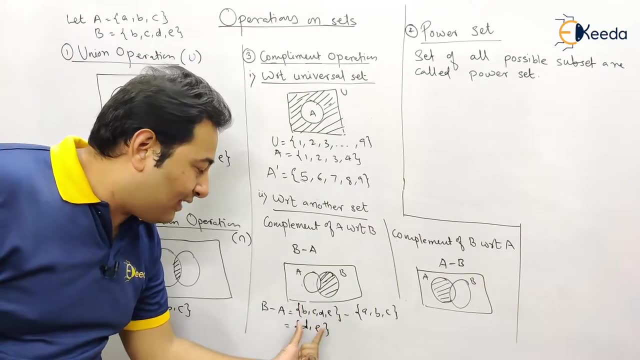 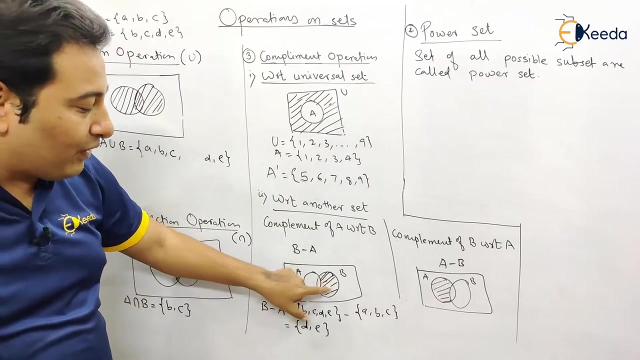 see here: B is common will be cancelled, C will be cancelled, B and C will be cancelled. will be left with D, E, Obviously, whatever. inside B, that will be a solution. See here. this A will not come into the solution part. see here. Therefore it is B minus A, So whatever. 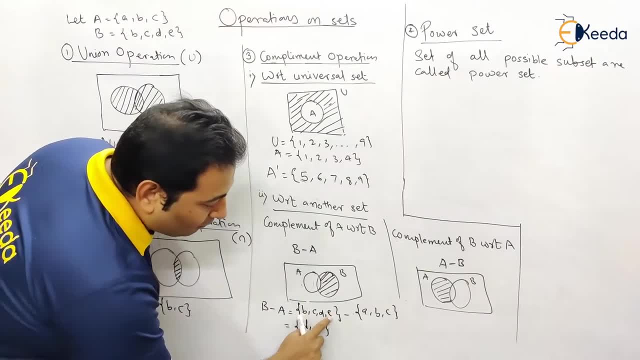 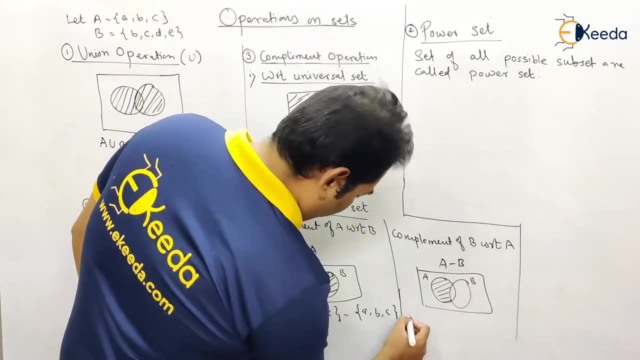 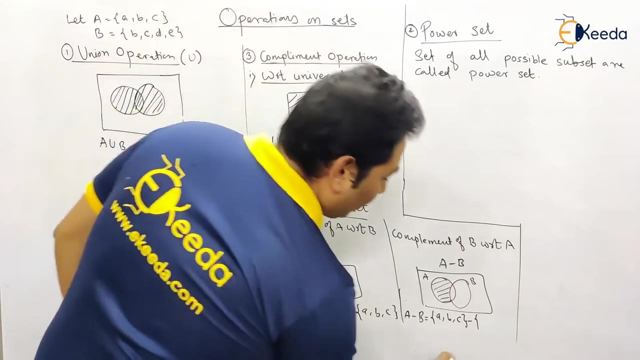 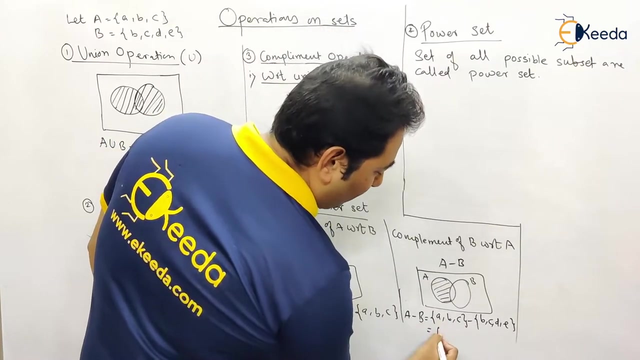 remaining in B. that will come into the solution part. So we're left with with de in the set b. therefore that will come into the solution part. here it is a minus b, so a minus b means abc minus bcde. if you subtract, see, this bc will be cancelled and will be left with a. so whatever with left with the. 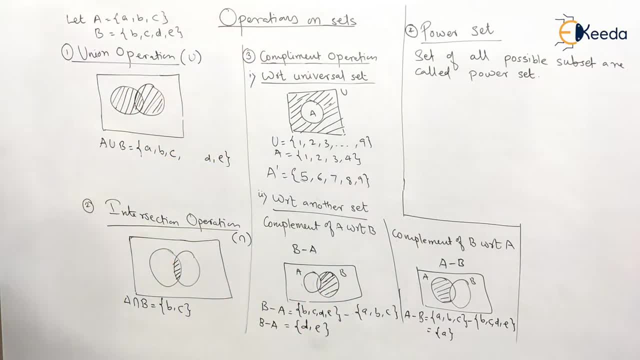 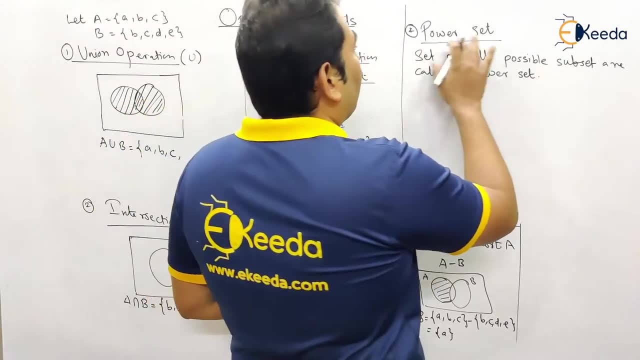 in the first set. that is your solution. so here it will be a. so this is your complement operation. so it can be with respect to universal set or it can be with respect to another set. next, the next operation is power set. power set means set of all possible subset are called power set. 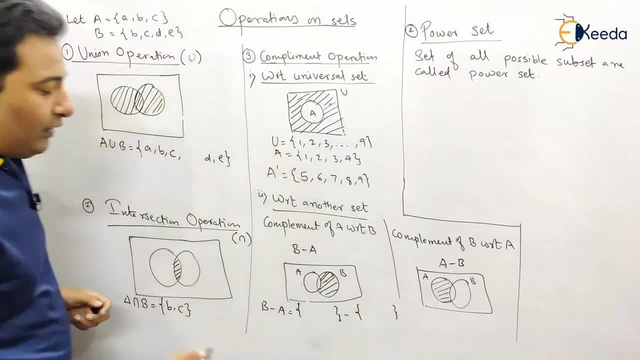 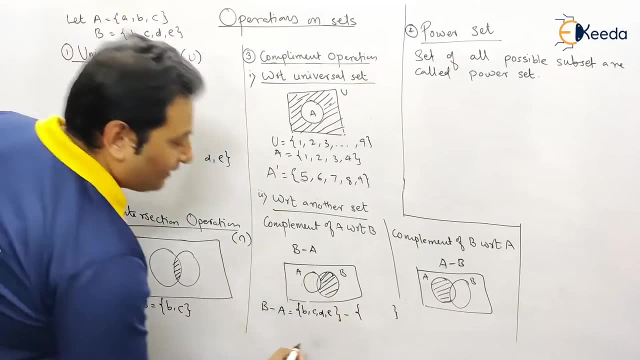 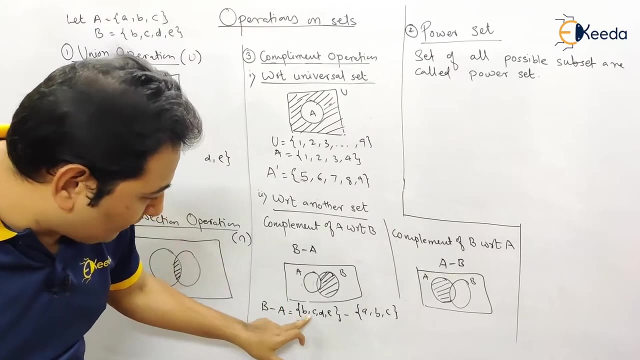 help of the same example. this example: if I'll write B minus a, please tell me what will be the answer from B. we going to subtract a simple�오. So if I subtract, what will be the result? Simply see here: B is common will be cancelled. 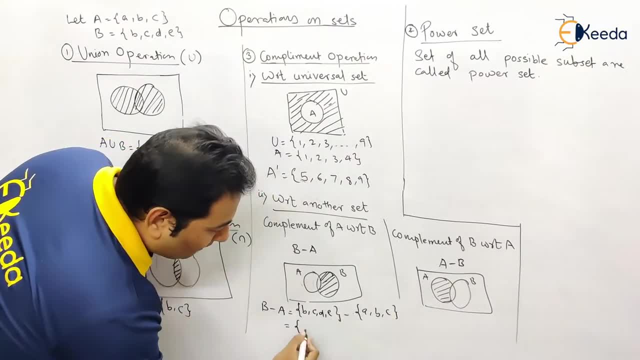 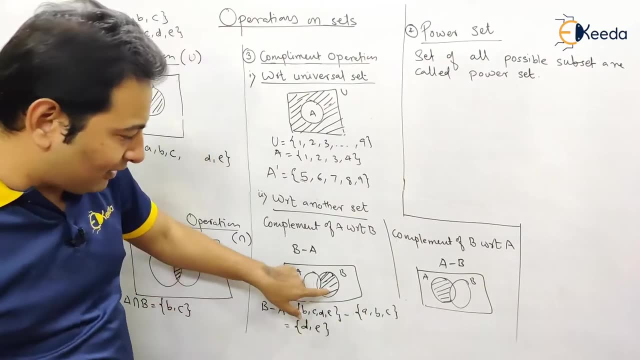 C will be cancelled. B and C will be cancelled. will be left with D, E, Obviously, whatever in set B that will be a solution. See here this: A will not come into the solution. part C: here Therefore it is B minus A. So whatever remaining in B that will come into the solution. 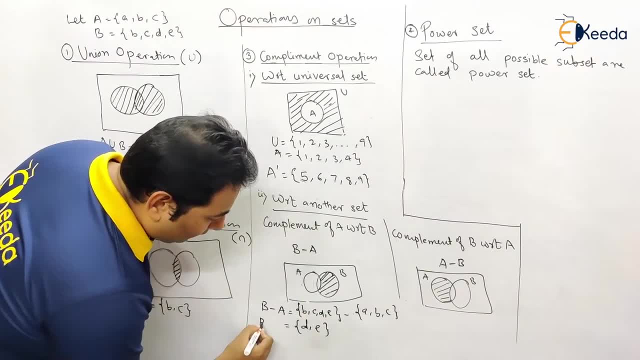 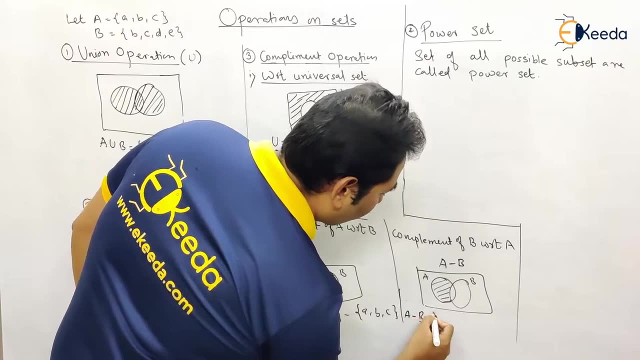 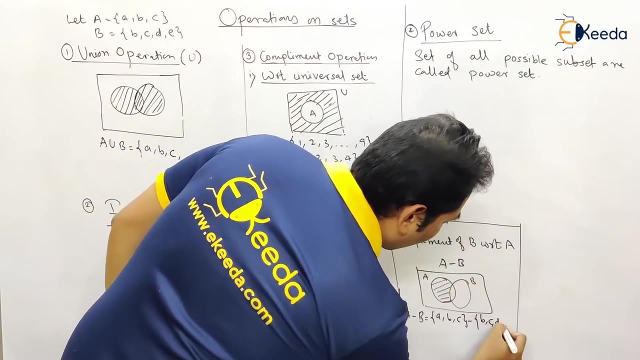 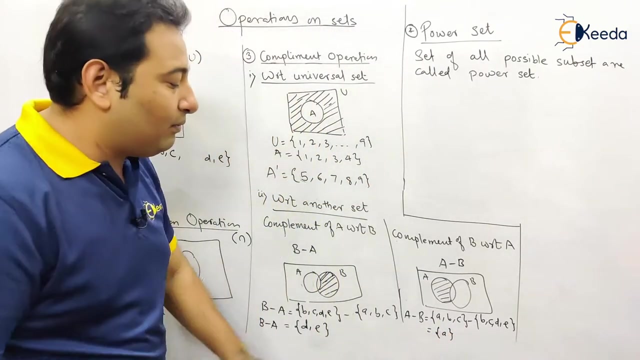 part. so we are left with DE in the set B. Therefore, that will come into the solution part. Here it is A minus B, so A minus B means BC minus DCE. if you subtract see this, BC will be cancelled and will be left with A. So whatever, we left with the in the first set. 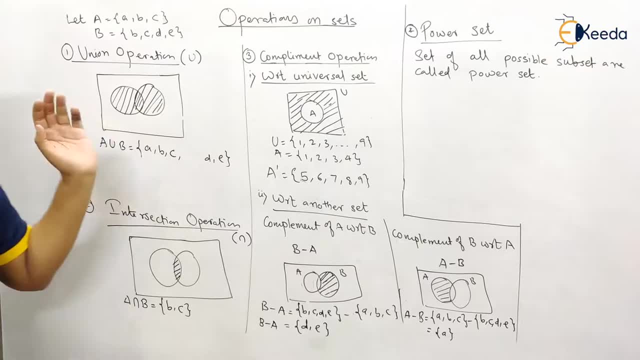 that is your solution. So here it will be A, So this will come into the solution part. Now, at that time, when we你想 to, will not, is your complement operation. so it can be with respect to universal set or it can be with respect. 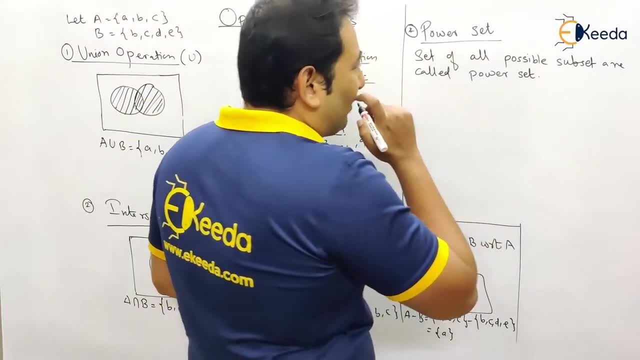 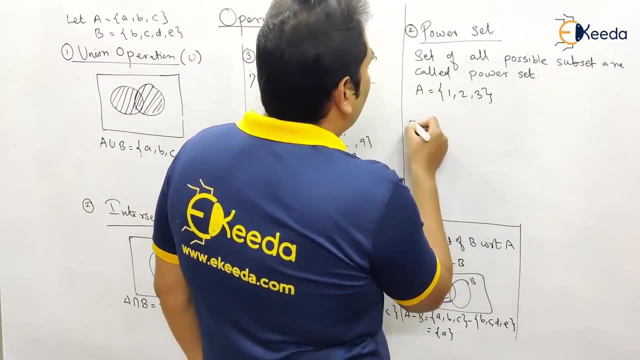 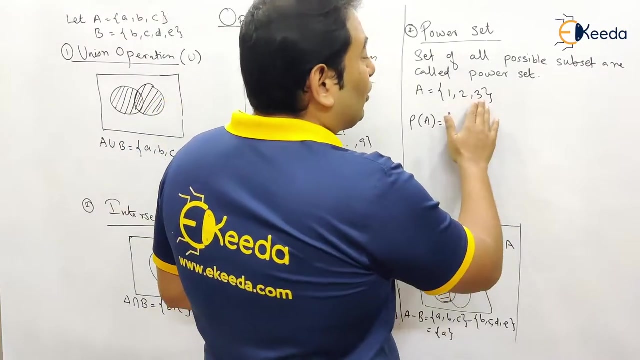 to another set next. the next operation is power set. power set means set of all possible subset are called power set. for example, suppose a is equal to 1, 2, 3. now what will be the elements in power set of a? yes, what will be the element in the power set of a? all the possible subset. please tell. 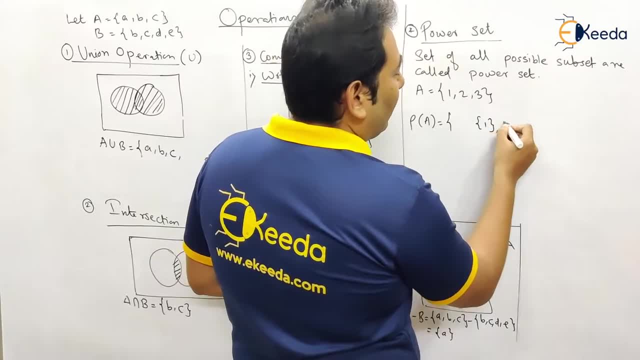 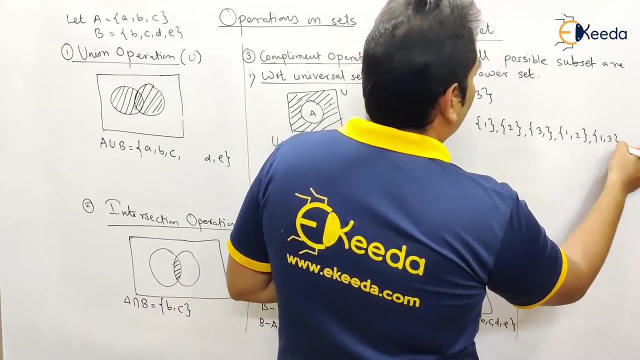 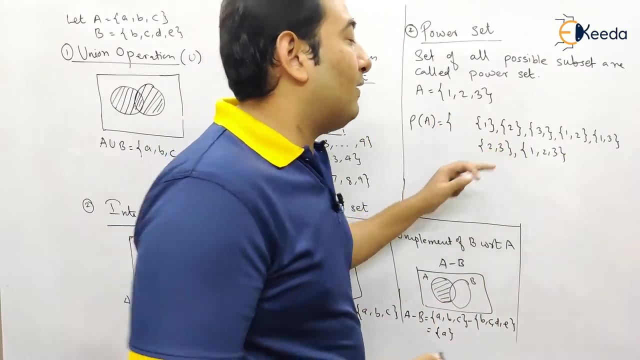 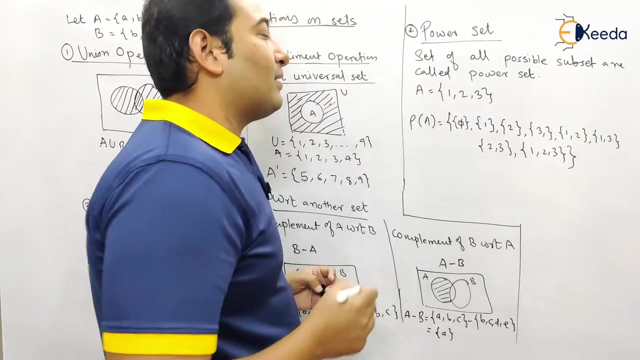 me. what are the possible subset? one. next possible subset: two, three. one, two, one, three, two, three. what else? one, two, three, because every set is a subset of itself. one more set: what is that? five? five means empty null set. null set is a subset of every set, so this is called power set. what do you know? 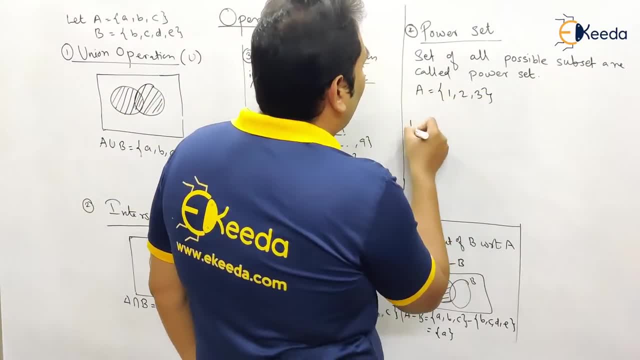 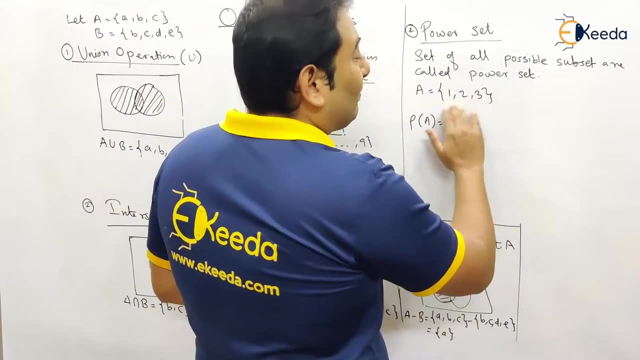 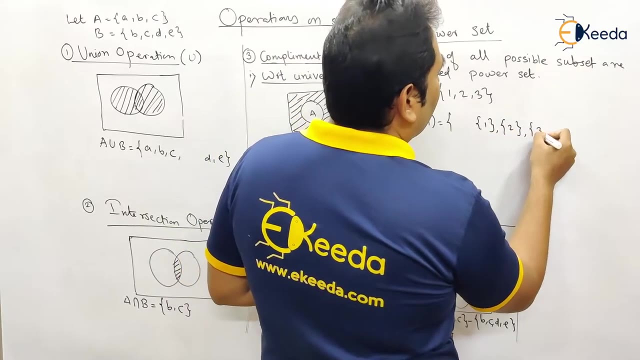 for example, suppose a is equal to one, two, three. now what will be the elements in power set of a? yes, what will be the element in the power set of a? all the possible subset. please tell me what are the possible subset one. next possible subset: two, three. 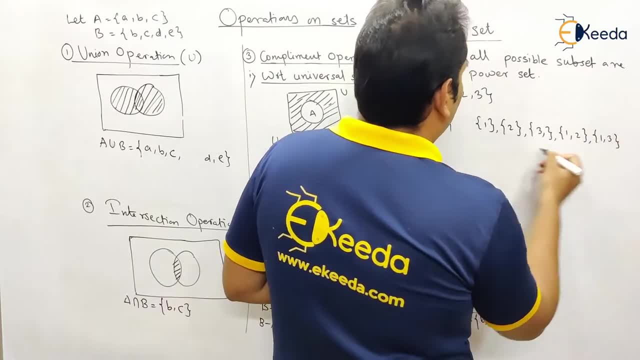 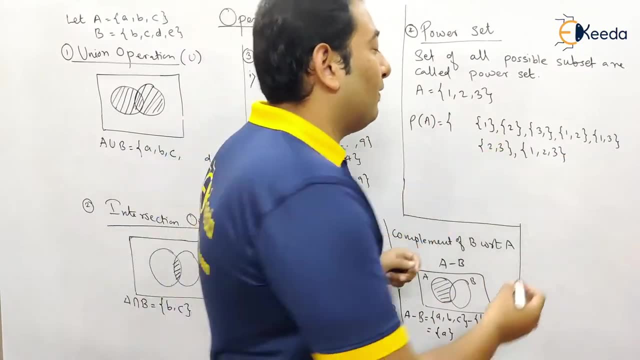 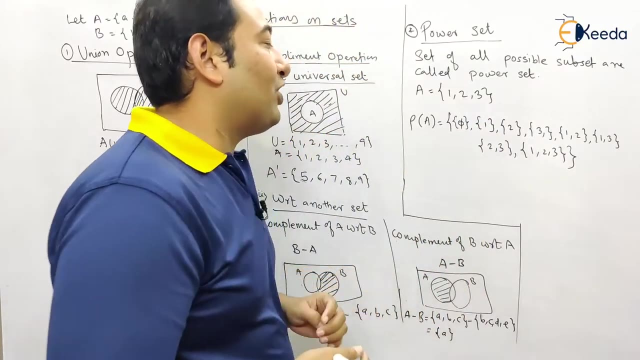 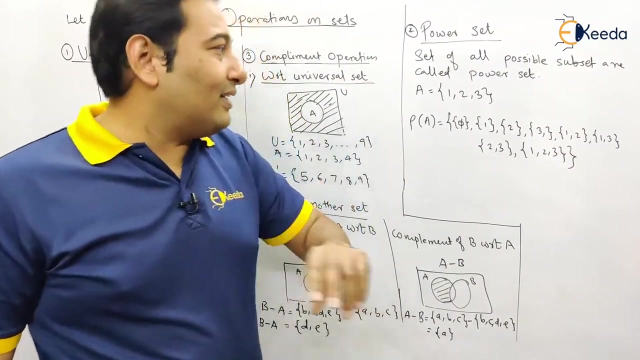 one, two, one, three, two, three. what else? one, two, three, because every set is a subset of itself. one more set. what is that? phi? phi means empty null set. null set is a subset of every set, so this is called power set. what do in my power set? set of all possible subset are called power set and it is represented by p of k. 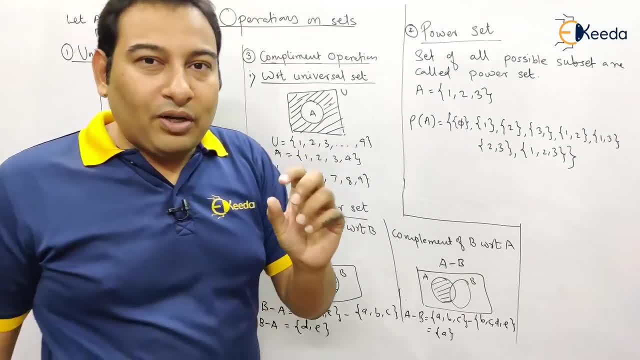 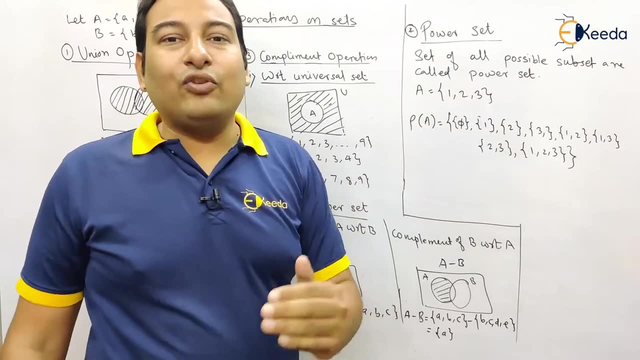 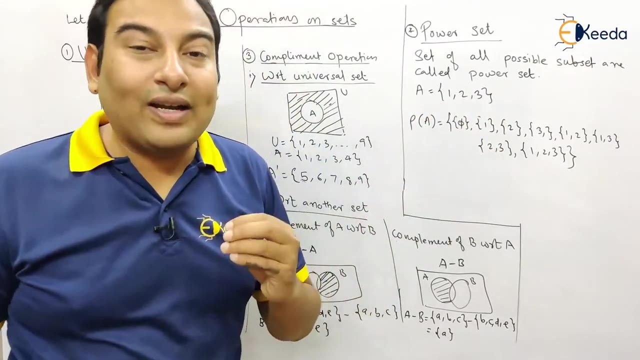 is this clear? now there is a very popular question that can be asked: how is rял in your limit set with different set of certain set elements? it can come as regard. you can ask else- variation in your limit set. again you can ask: and the a common above the element which is in the power set? 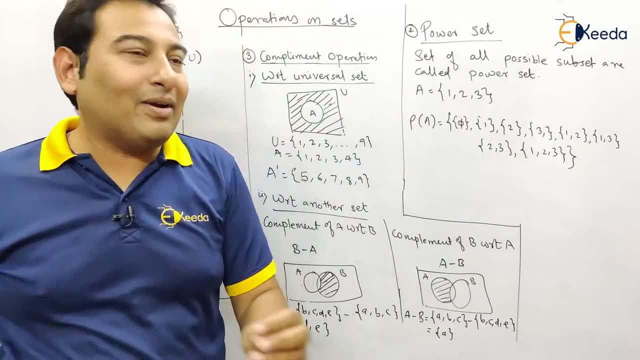 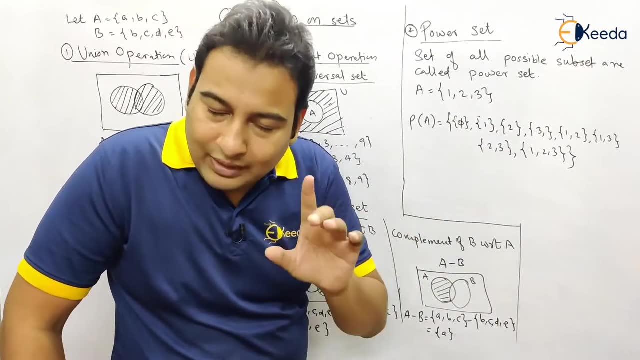 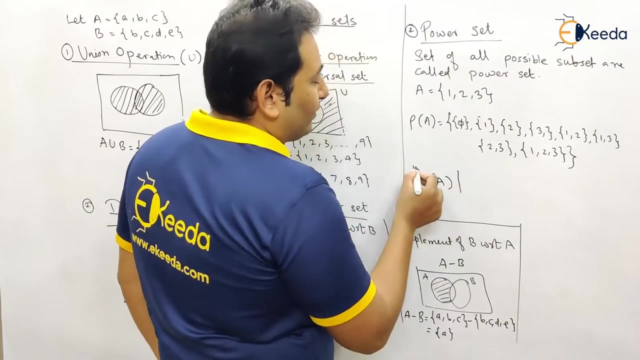 i mean this set of elements. this is a set- will be given and you need to find out the number of elements in power set. here, 123 is given and it is asked to find it out the number of elements in power and the formula is: see. this is called cardinality. it indicates number of elements. so this is your. 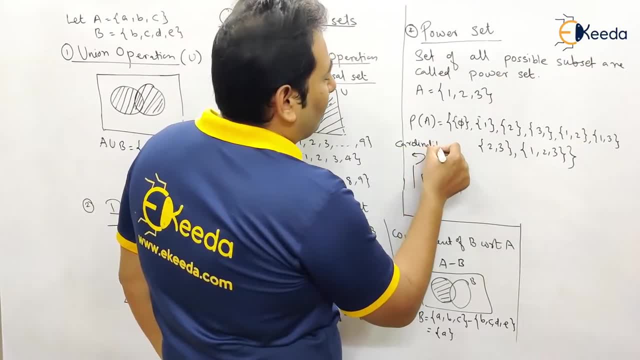 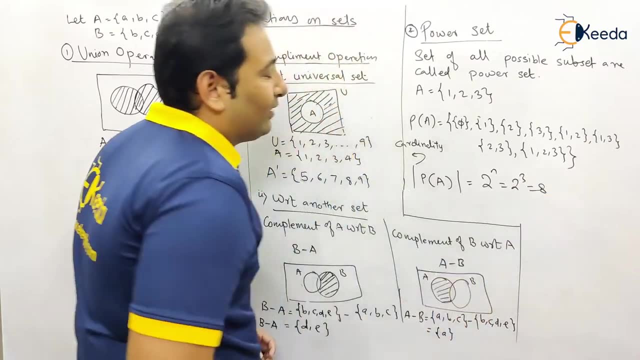 cardinality and the formula is 2 raised to n, so that is 2 cube is equal to 8, so there are 3 elements in a set, 2 cube 8. so there will be 8 elements in a power set. so very important formula. 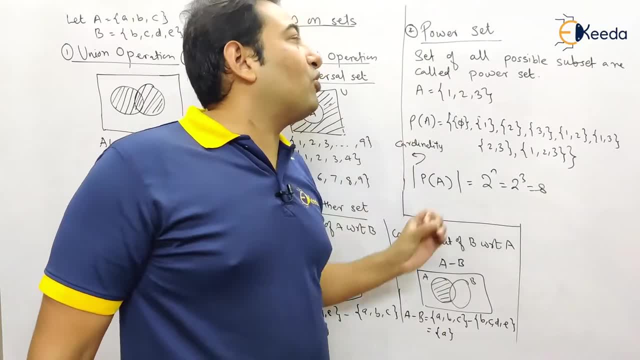 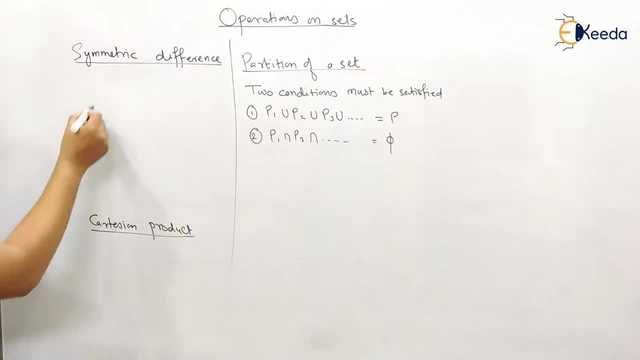 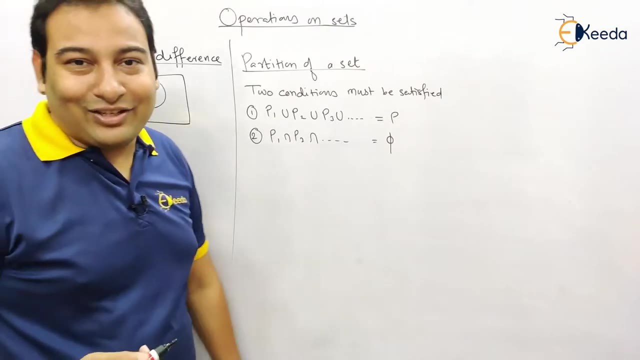 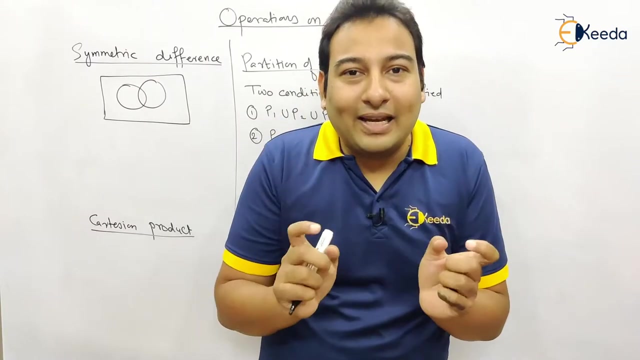 that you need to remember. so this is the concept of power set. set of all possible subsets are called power set. now we'll discuss the next operation, that is, symmetric difference. symmetric difference mean opposite to intersection. in intersection, what we do? we take common elements. in case of symmetric difference, we'll leave common elements and we're going to consider the. 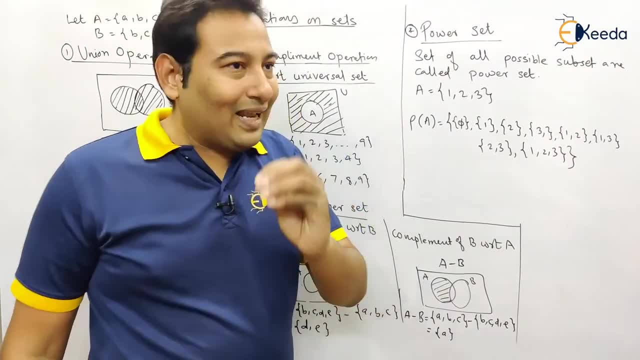 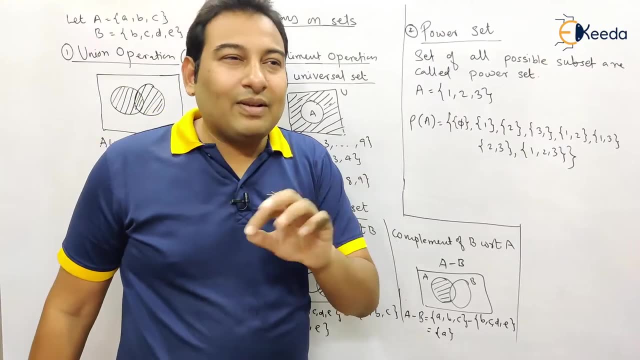 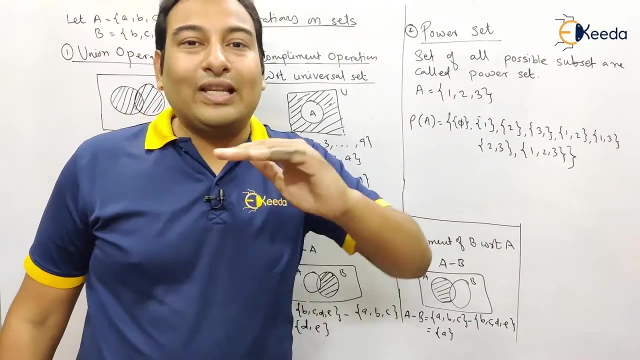 power set. set of all possible subset. subset are called power set and it is represented by p of k. is this clear? now there is a very popular question that can come as an mcq in your paper or that can come in a great exam. a set will be given and you need to find it out: the number of elements in power set. 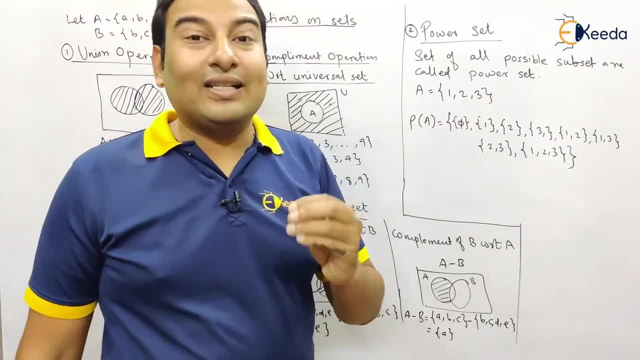 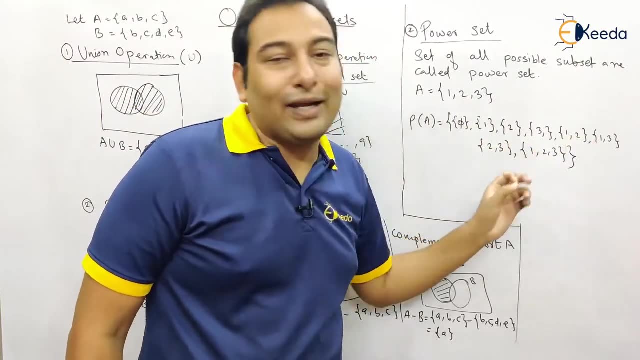 see here: 1, 2, 3 is given and it is asked to find it out the number of elements in power set. see how many elements are there: 1, 2, 3, 4, 5, 6, 7, 8. so there are 8 elements, if there. 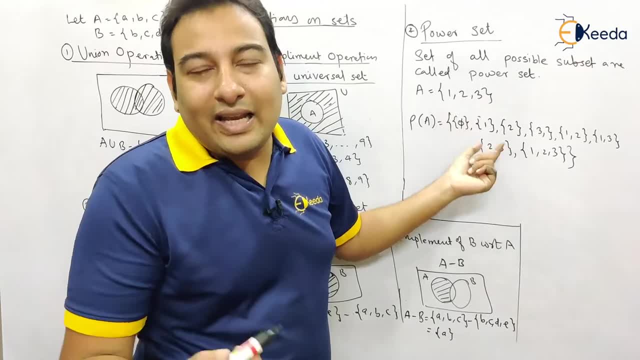 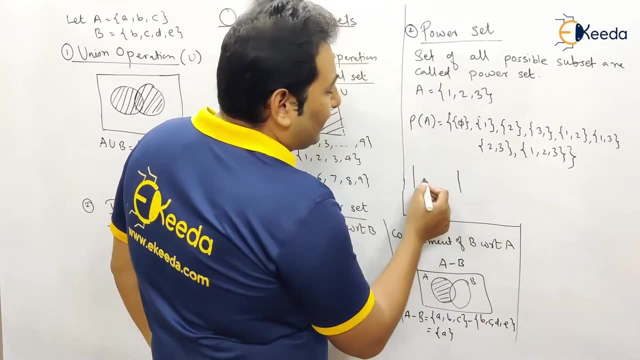 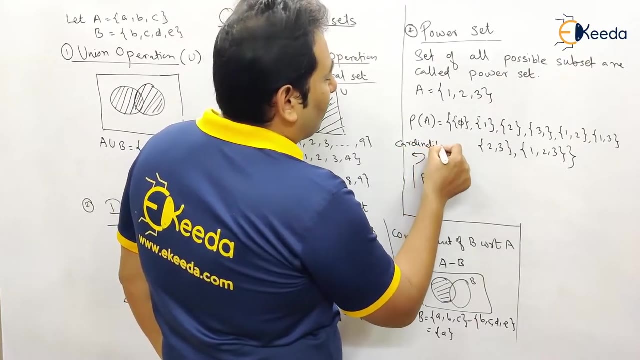 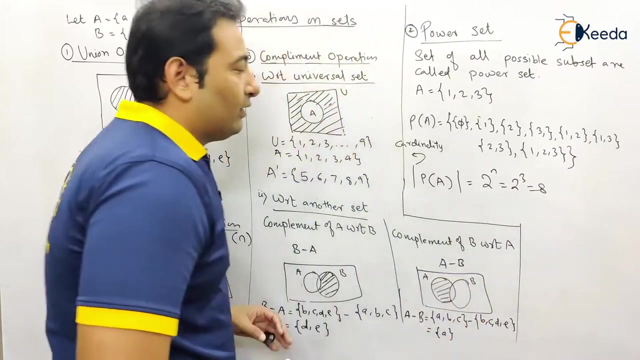 are 3 elements in a set A, there will be 8 elements in power set. so is there any formula? yes, there is a formula and the formula is: see, this is called cardinality. it indicates number of elements. so this is your cardinality. and the formula is 2 raised to n, so that is 2. cube is equal to 8, so there are 3 elements. 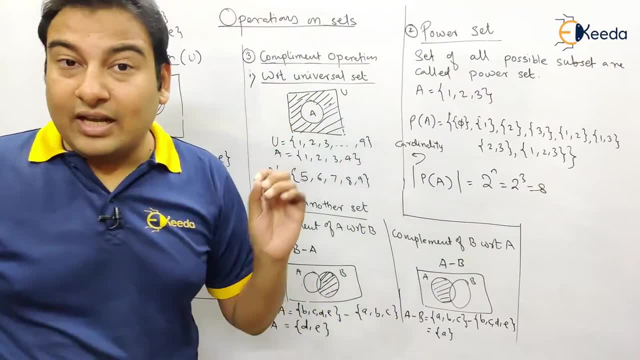 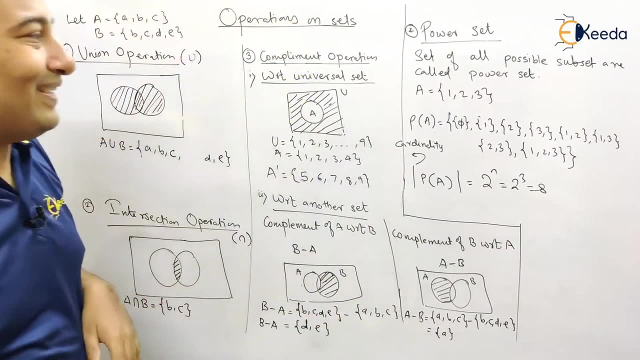 in a set 2 cube 8. so there will be 8 elements in the power set back. So very important formula that you need to remember. So this is the concept of power set. Set of all possible subsets are called power set. 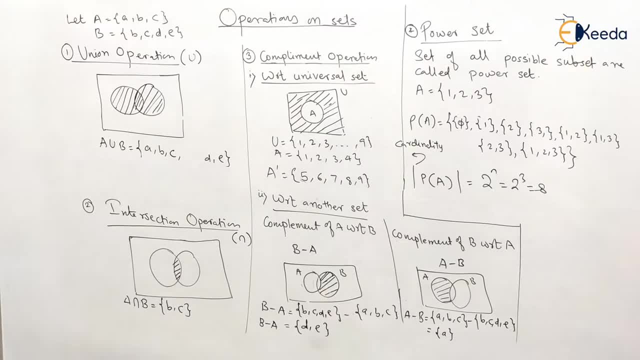 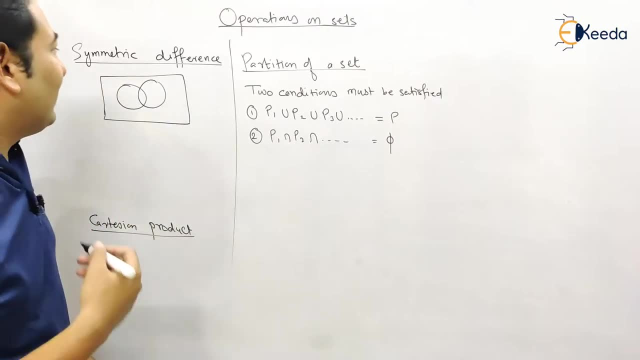 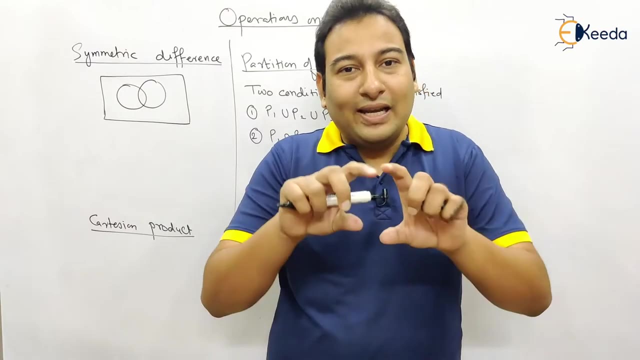 Now we'll discuss the next operation, that is, symmetric difference. Symmetric difference mean opposite to intersection. In intersection, what we do, We take common elements. In case of symmetric difference, we'll leave common elements and we're going to consider the remaining elements. 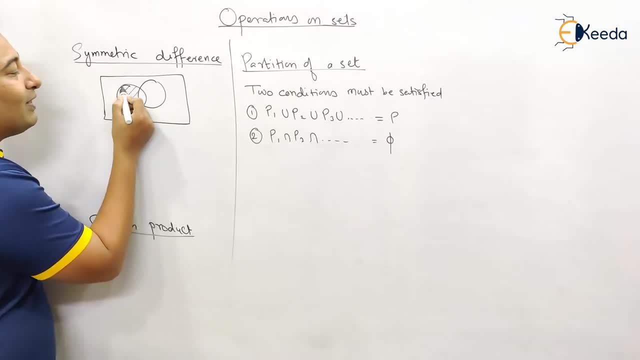 See, this is your common part, that is your intersection. In case of symmetric difference, we're not going to consider the common elements. We'll take the same example. Let's say A is equal to ABC and let's say B is equal to BCDE. 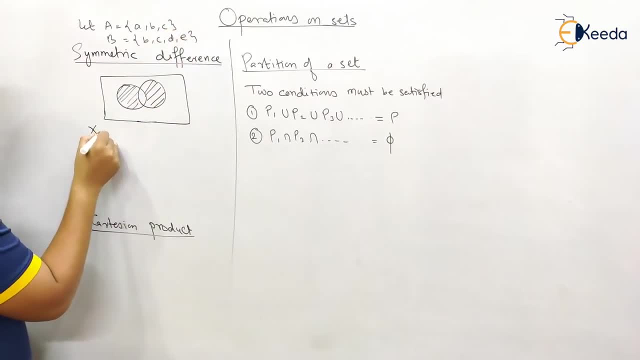 Symmetric difference is also called XOR operation or ring sum, So remember the names and it will be simply A, XOR, B or ring sum, Or symmetric difference. So we're going to leave the common elements Here. the BC is common element. 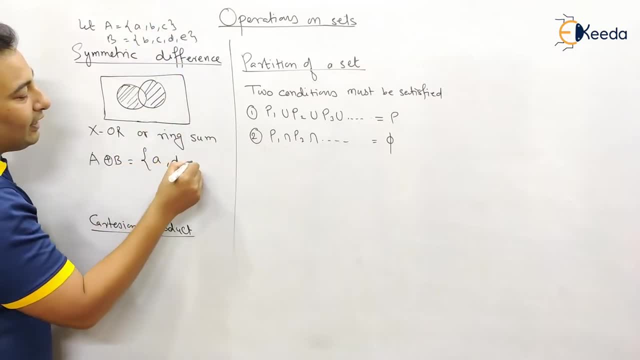 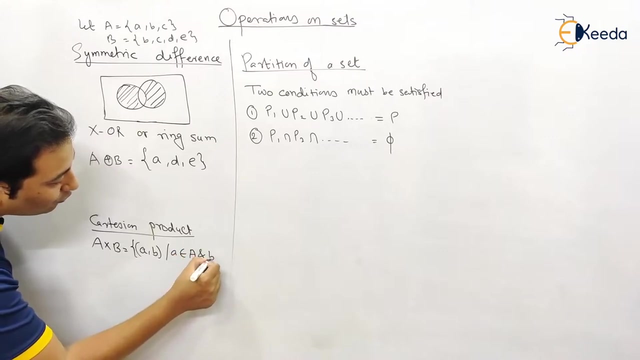 So we're going to leave it and we'll be left with what? A, D and E. So this is your symmetric difference. What is the next Cartesian product? Next operation is Cartesian product? Very simple operation: A X, B is equal to A- B, such that A belongs to A and B belongs to B. 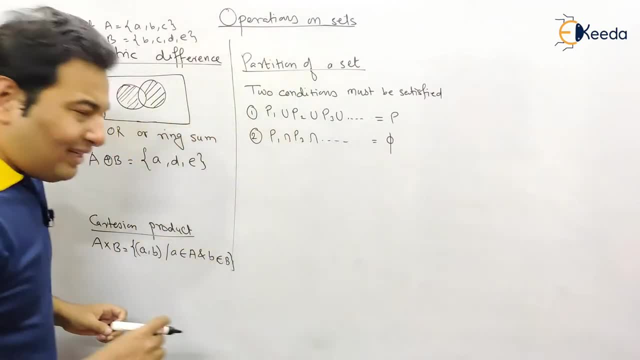 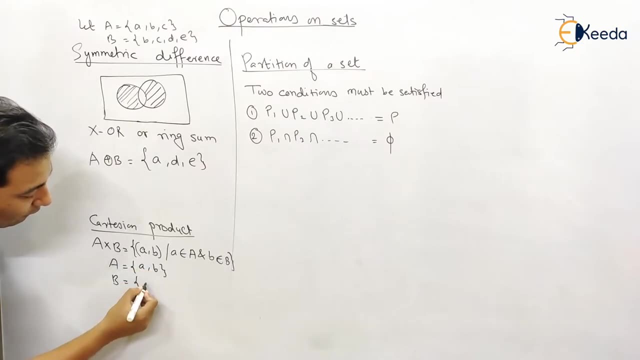 So this is the definition of a Cartesian product, And it is simply multiplicated. There is no multiplication, nothing else. See, suppose in A we have A B, and suppose in B we have, let's say, 1, 2.. 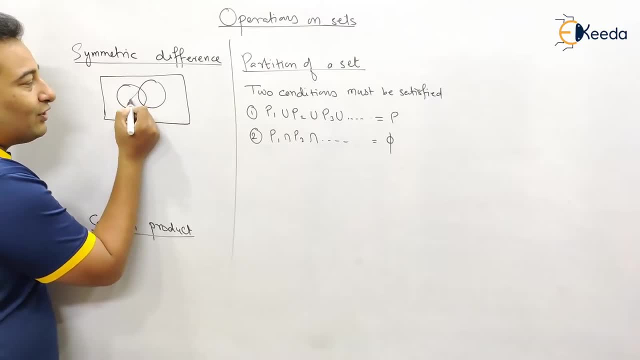 remaining elements. see, this is your common part, that is your intersection. in case of symmetric difference, we're not going to consider the common elements. we'll take the same example. let's say a is equal to abc and let's say b is equal to b, c, d, e, symmetric. 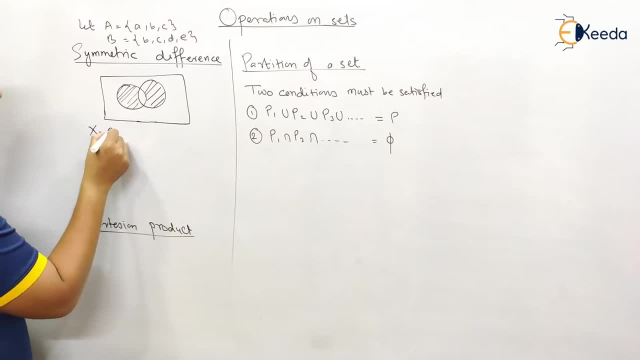 difference is also called xor operation or ring sum, so remember the names and it will be simply a, xor, b or ring sum, or symmetric difference. so we're going to leave the common elements here. the bc is common element, so we're going to leave it and we'll be left with what. 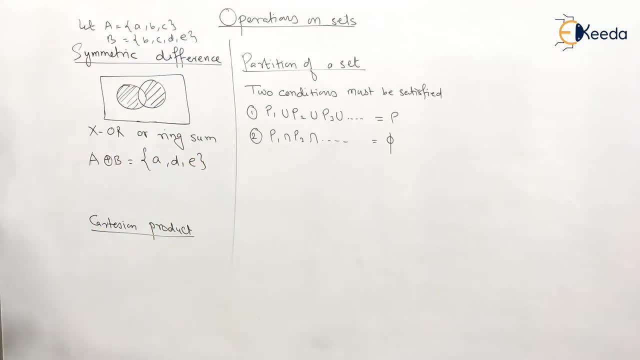 a, d and e. so this is your symmetric difference. what is the next cartesian product? next operation is cartesian product. very simple operation: a cross b is equal to a, comma b, such that a belongs to a and b belongs to b. so this is the definition of a cartesian product and it is simply multiplication. 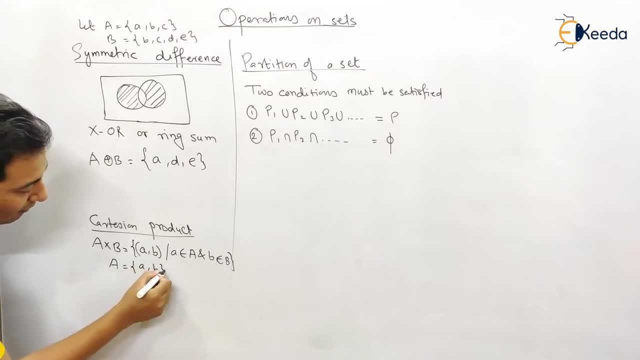 nothing else. see, suppose in a we have a comma b and suppose in b we have, let's say, one comma two. so if i'll write a cross b, it's just a multiplication: a comma one, a comma two, b comma one and b comma two. it's simple multiplication: a comma one, a comma two, b comma one and b comma two. and likewise, if i'll 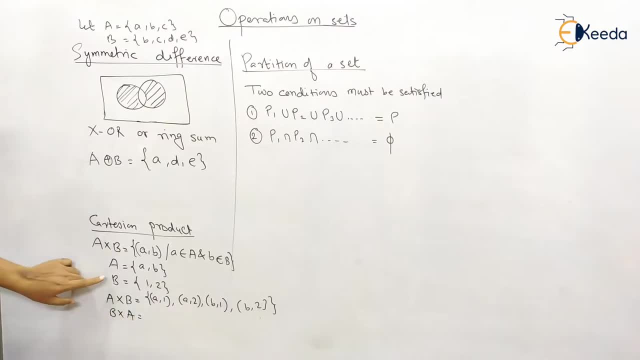 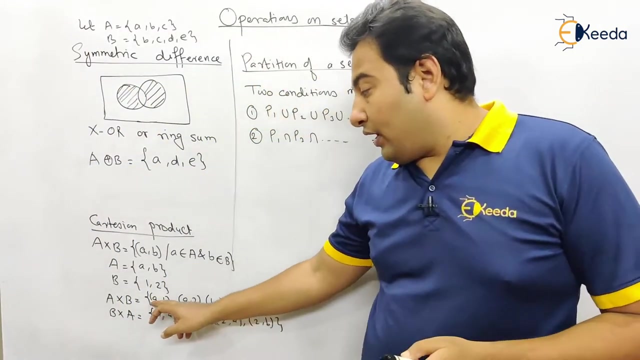 write b cross a, so in that case b will be multiplied to it. so that is one comma a, one comma b, two comma a and two comma b. so this is your b cross a. here order is very important. that means a comma one is different from one comma a. now what do you? 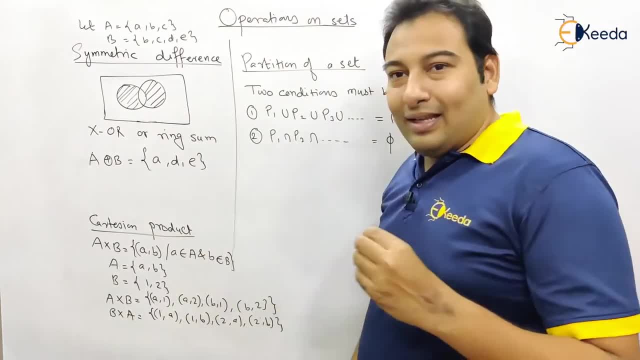 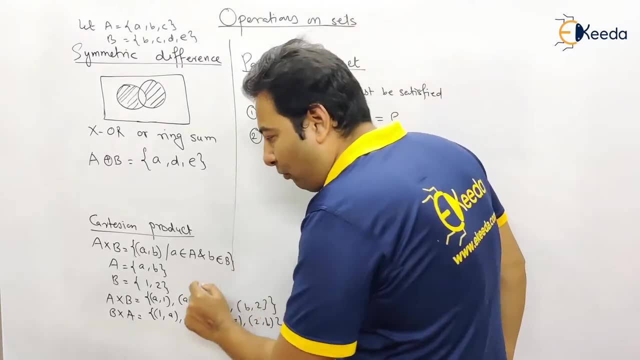 mean by this definition. this definition is very important. soon, uh, in coming videos, we'll discuss problem based on that, so it's very important. and what does the definition indicate? see, it's very important. first element: a belongs to the first set, so it's very important. and what does the 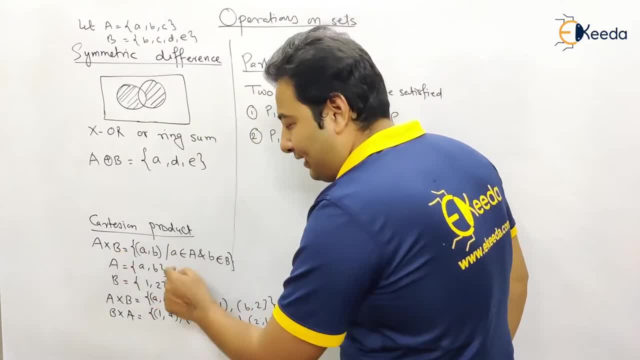 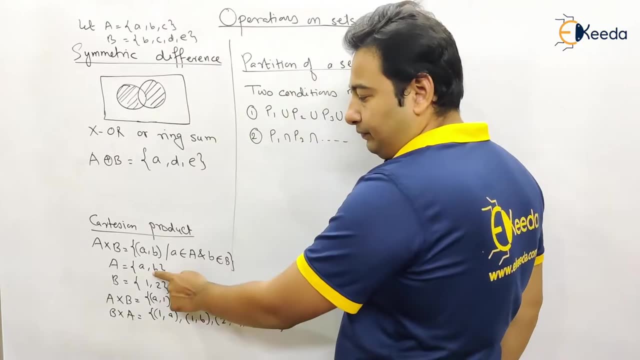 definition indicate, see here. it's always a set of elements and it should not be more than a set. and this element belongs to the second set, see here. you take any example. let's say this: b belongs to the a and one belongs to b, see here. so the first element always belongs to the first set and the 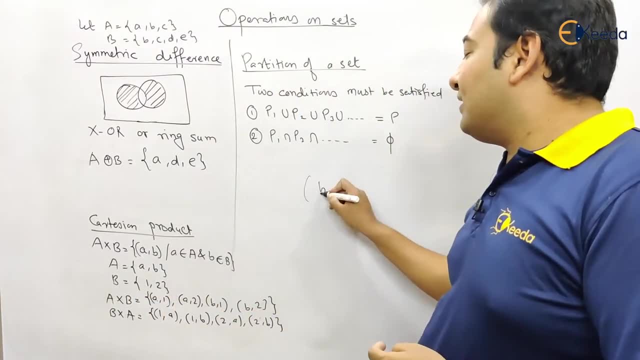 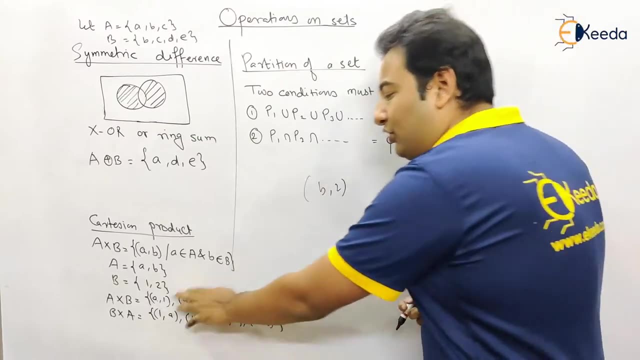 second elements always belongs to the second set. so randomly, if i'll say b, comma two, please tell me will this term will be in a cross b or b cross a? don't check this. see here this b is in capital a, b and this will be in a cross b. okay, because b is minor or b single, so this is not a быть inив. 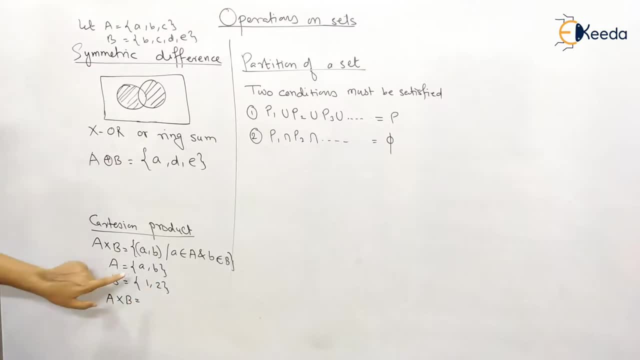 So if I write A X, B, it's just a multiplication A 1, A 2, B 1 and B 2.. It's simple multiplication: A 1, A 2, B 1 and B 2.. 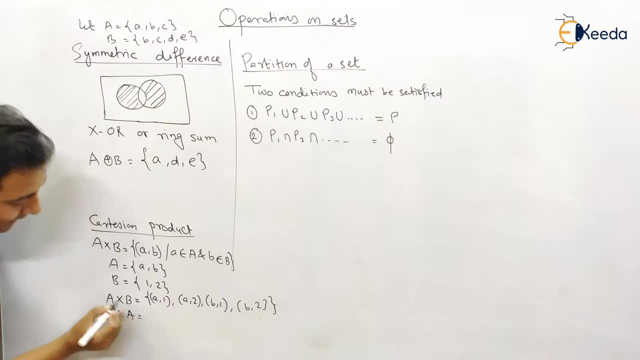 And likewise, if I write B X A, So in that case B will be multiplied to A, So in that case B will be multiplied to A, So that is 1, A, 1, B, 2, A and 2, B. 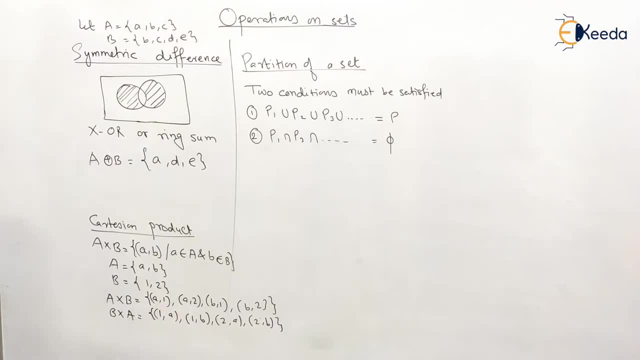 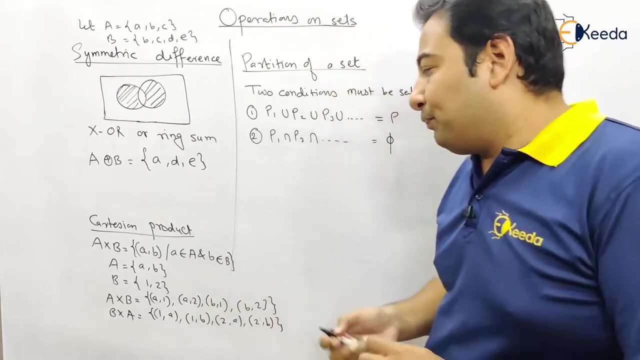 So this is your B, X, A. Here order is very important. That means A, 1 is different from 1, A. Now what do you mean by this definition? This definition is very important. Soon in coming videos. 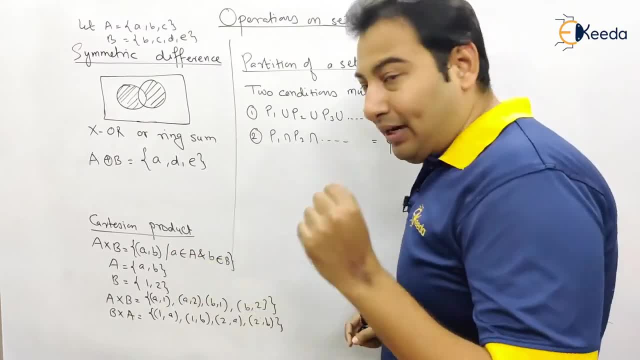 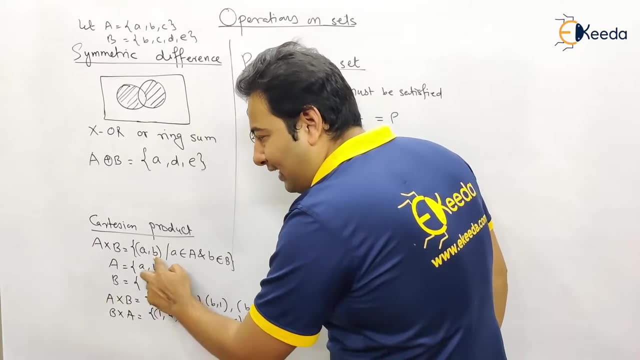 we'll discuss problem based on that. So it's very important. And what does the definition indicate? See, it's very important. First element A belongs to the first set and this element belongs to the second set. See, here You take any example. 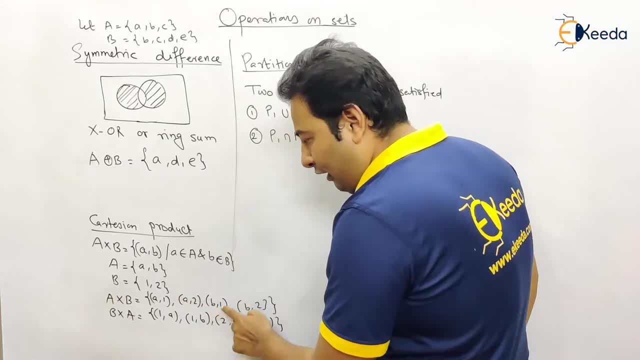 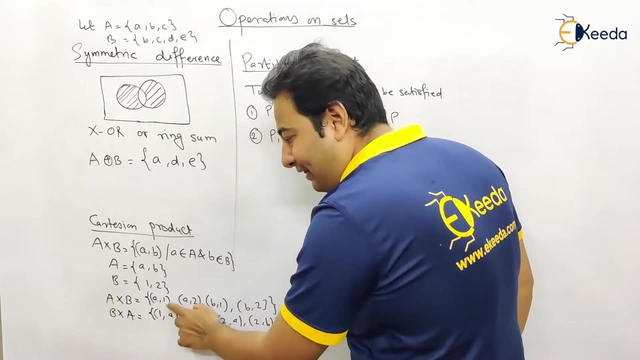 Let's say this: B B belongs to the A and 1 belongs to B, See here. So the first element always belongs to the first set and the second element always belongs to the second set. So randomly, if I'll say B 2.. 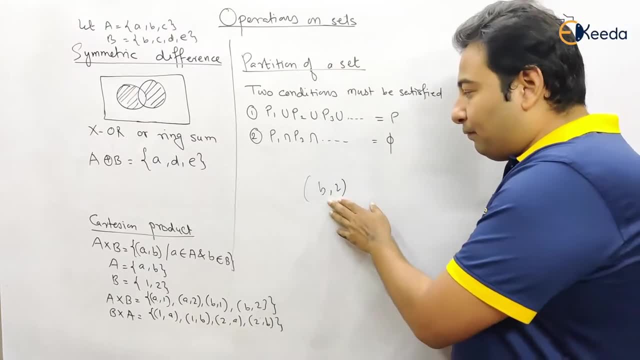 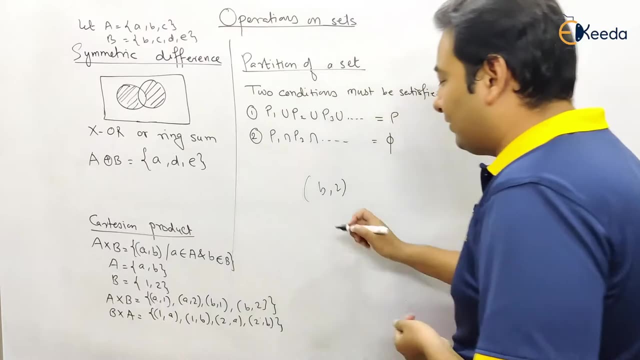 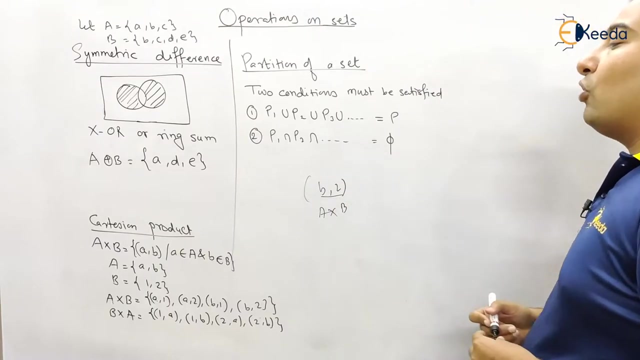 Please tell me will this term will be in A X B or B X A. Don't check this. See, here This B is in capital A, So this is A X. this 2 is in set B, So therefore B 2 must belong to A X B. 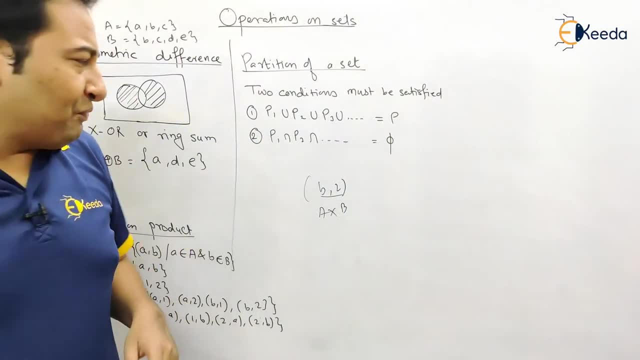 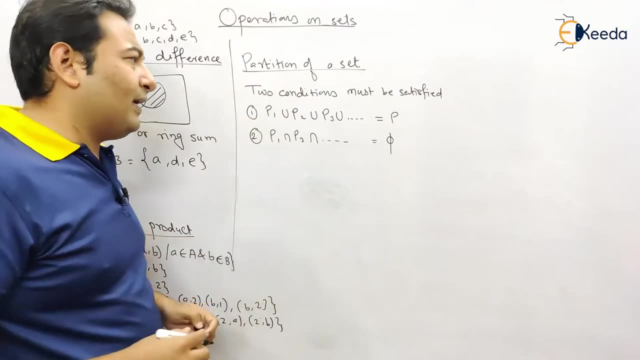 So this is very important. definition: Cartesian product. Okay, Let us move on and let us discuss the next concept, that is, partition of a set. It's very simple concept. again, Two conditions must be satisfied, So let me write it down an example. 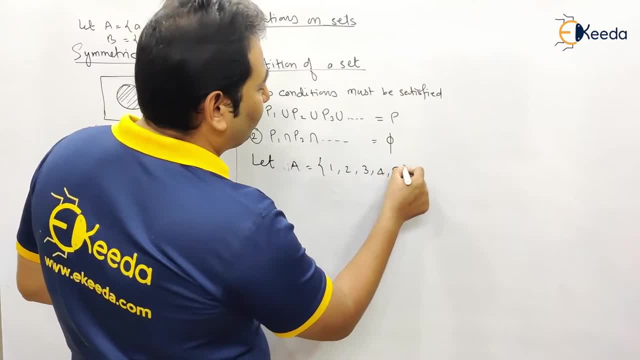 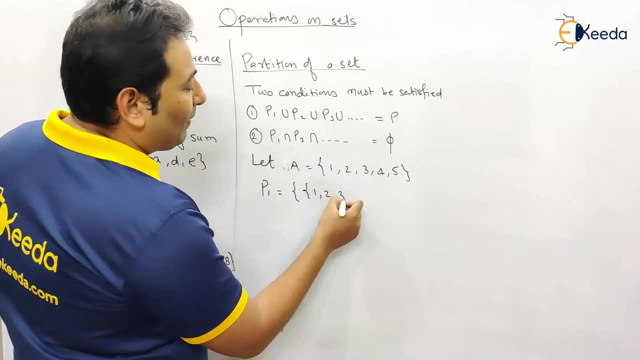 Let's say A is equal to 1,, 2,, 3,, 4 and 5.. Now I'm going to write it down: few sets that we're going to check whether they are a proper partition or not. I'll tell you how to check. 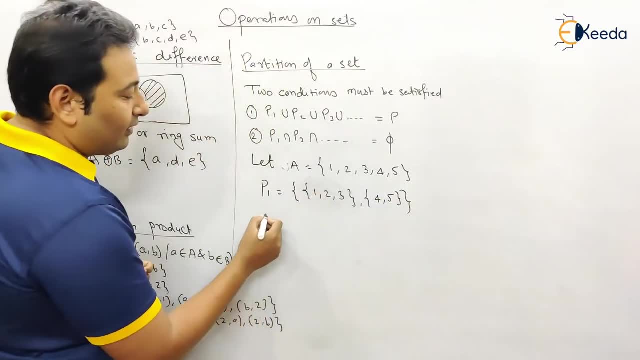 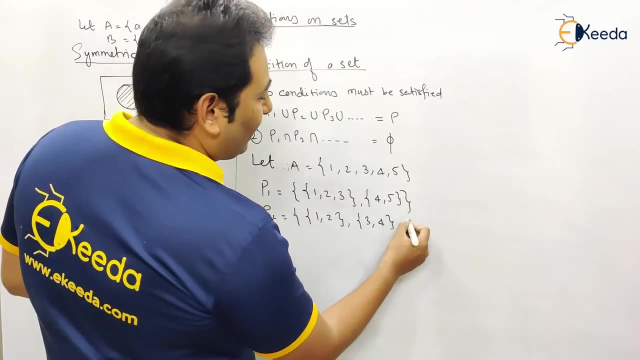 So don't worry about that. So this is the first set. We're going to check whether it's a partition or not. This also can come in the exam MCQ. There will be few sets given and it may ask to check. 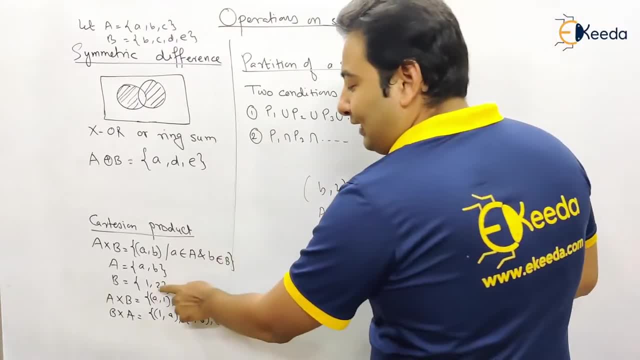 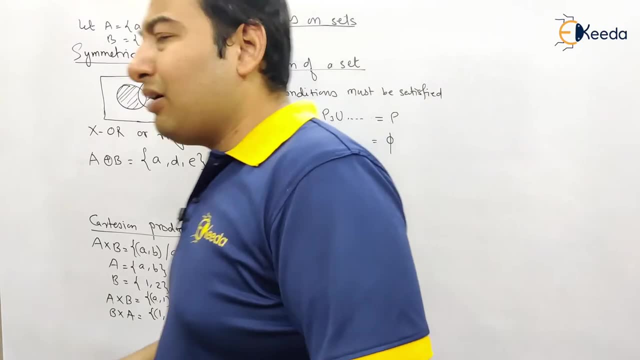 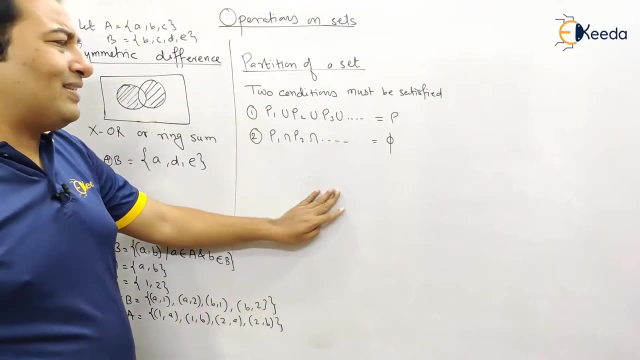 so this is a cross, this two in said b. so therefore b comma two must belong to a cross b. so this is very important. definition: cartesian product. okay, let us move on and let us discuss the next concept, that is, partition of a set. it's very simple concept. again, two condition must be satisfied. 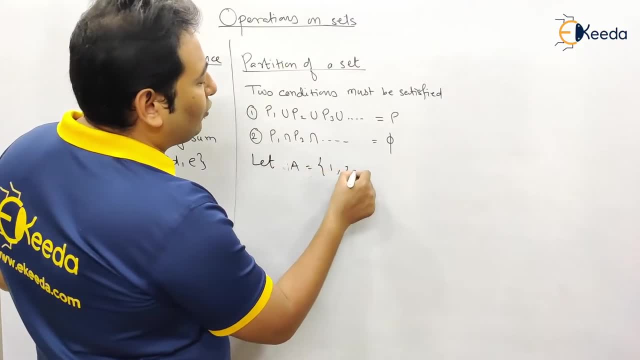 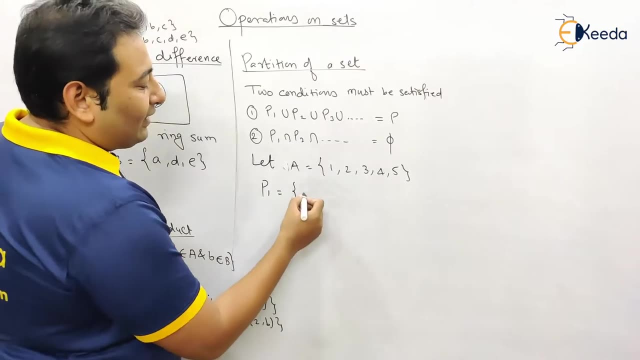 so let me write it down. an example. let's say a is equal to 1, 2, 3, 4 and 5. now i'm going to write it down, few sets that we're going to check whether they are a proper partition or not. i'll tell you. 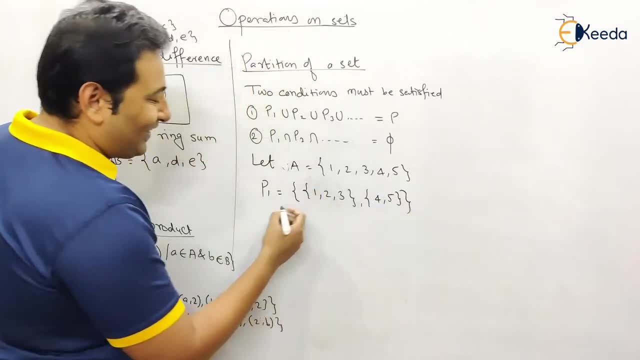 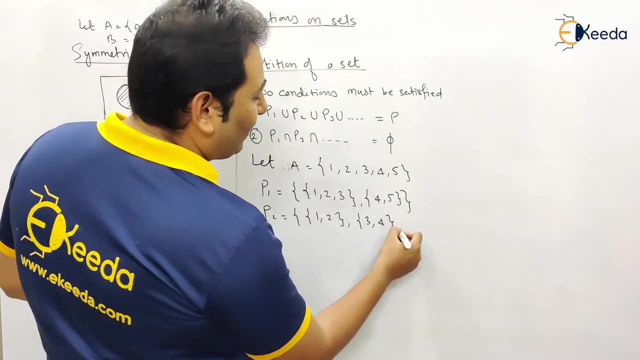 how to check, so don't worry about that. so this is the first set. we're going to check whether it's a partition or not. this also can come in the exam mcq. there will be few sets given and it may ask to check whether which one is partition and which one is not a partition. 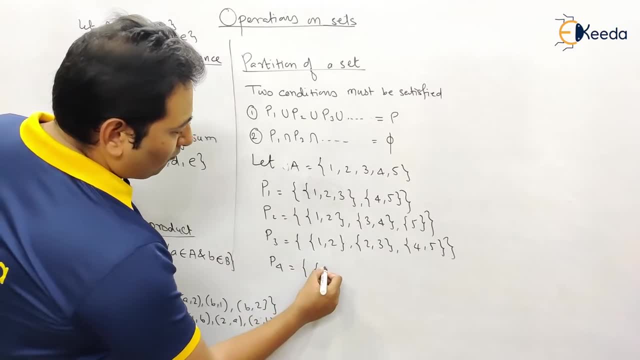 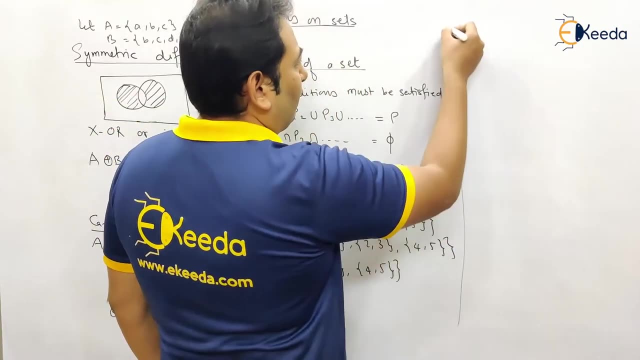 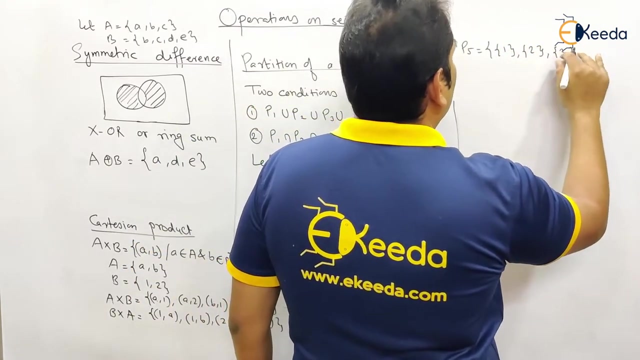 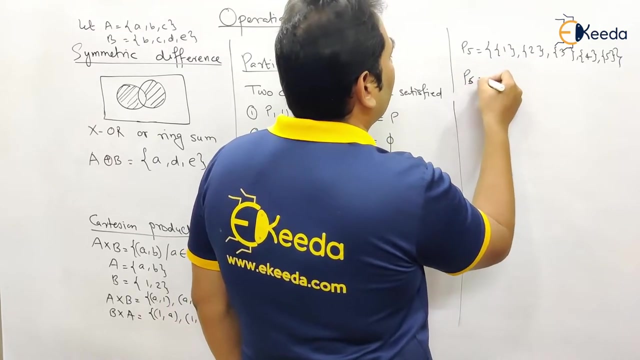 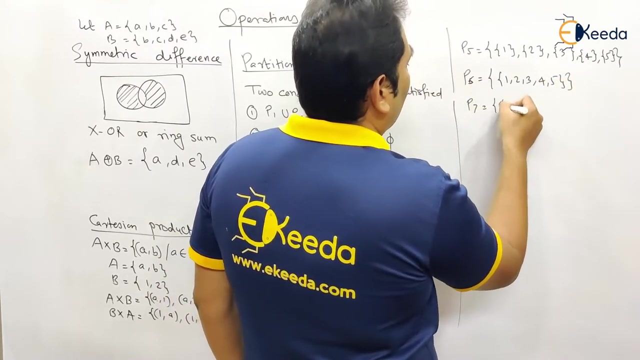 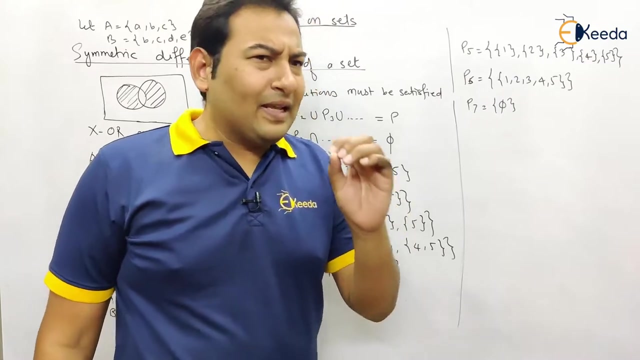 this is my third set. this is the fourth one. i'm just writing down the random example so it can. anything can come in the exam. so these are the seven examples that i've taken. now we're going to check which one are the proper partition or not. there should be two condition that should be satisfied for a set to be partition. 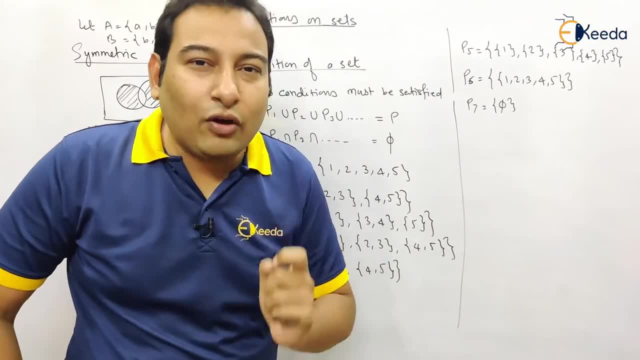 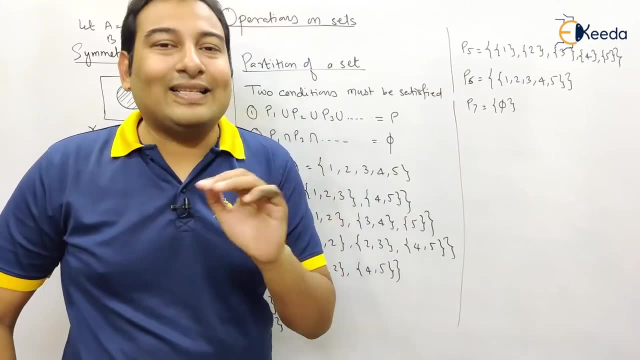 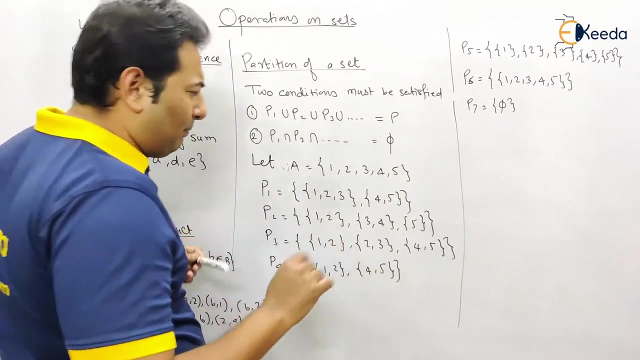 and the first condition is: if you take union of all it wish, if you take union of all, we should get the original set. and the second condition is: if you take intersection of any two set, we should get five. let us check what this exactly mean. it's very simple, see. 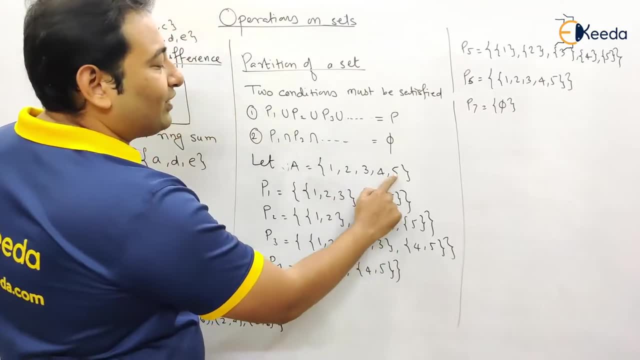 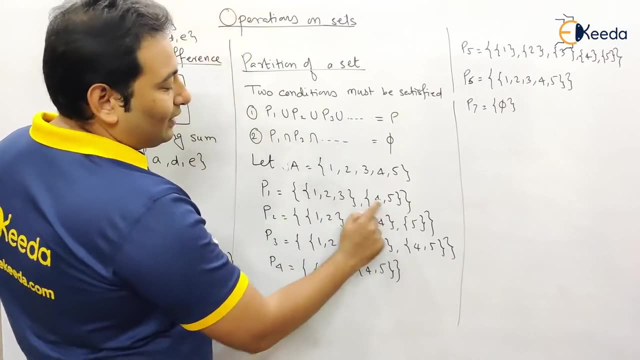 if you thank union of these two sets, you should get the original set. are you getting on this first condition, P1. P2.. P3 means this. so if you take union of these two sets- one, two, three, four, five- you are getting the original set. and the second condition is: 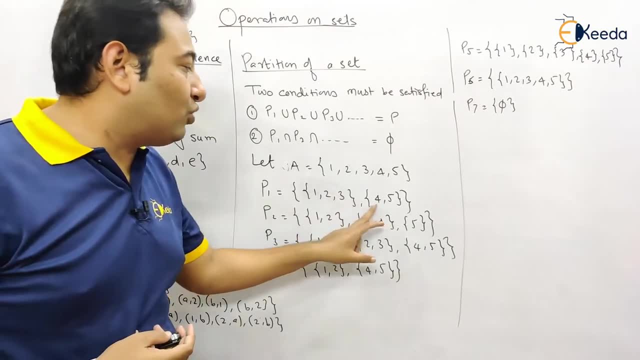 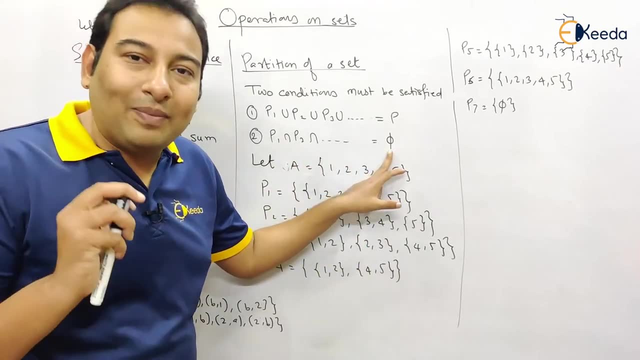 there should be anything common between the two sets. so if u take the union of these two, you'll get one, two, three, four, five, and there's nothing common. if you take the intersection, there should be nothing common. so both the condition are satisfied. 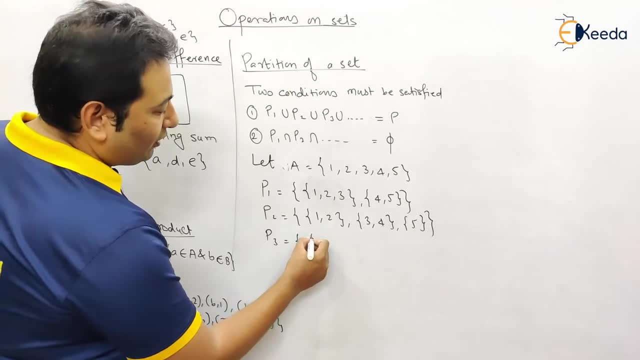 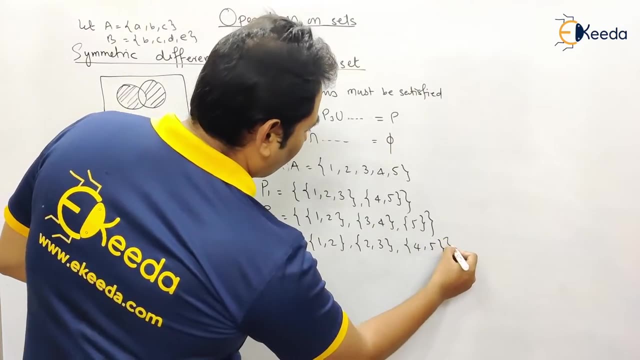 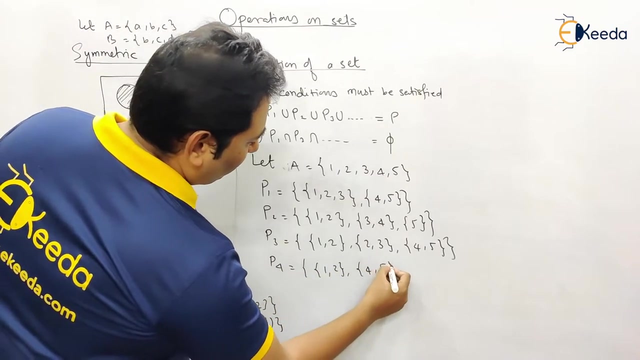 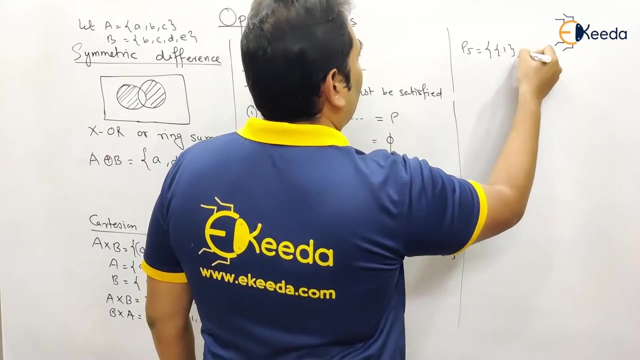 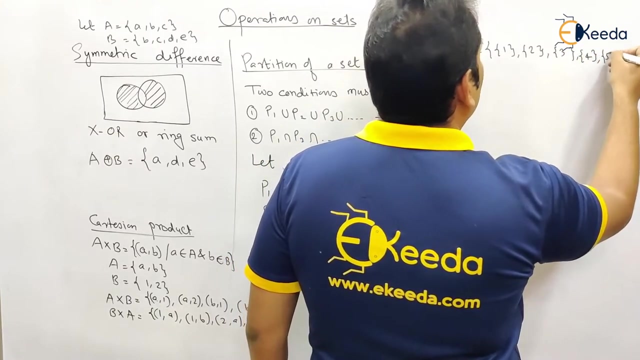 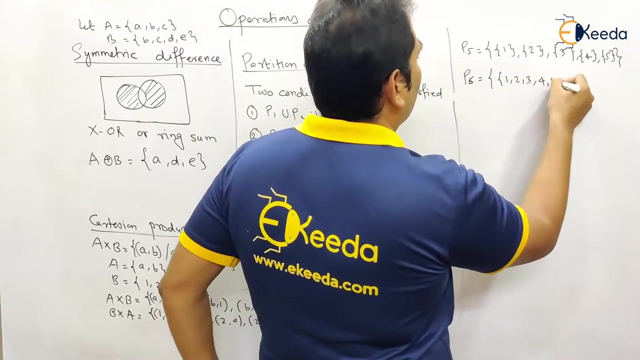 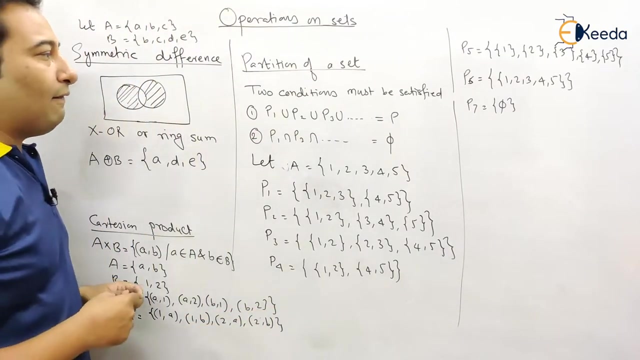 whether which one is partition and which one is not a partition. This is my third set. This is the fourth one. I'm just writing down the random example, So it can anything can come in the exam. So these are the seven examples that I've taken. 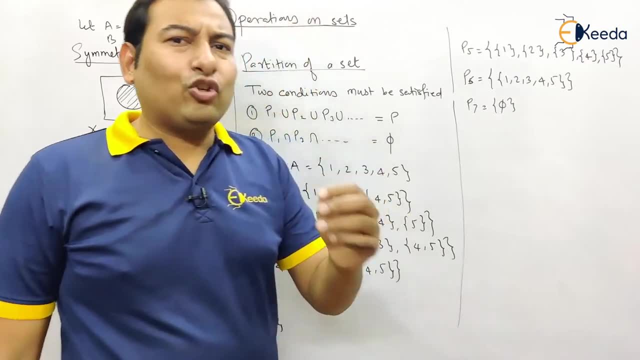 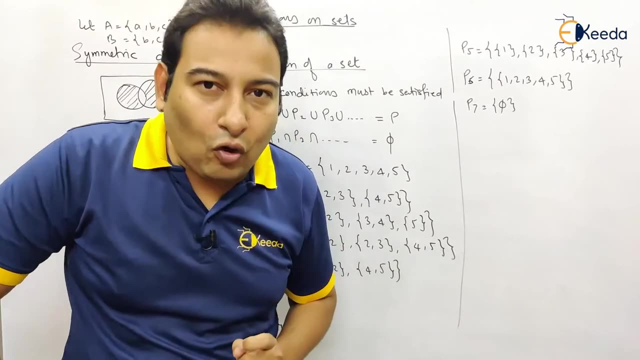 Now we're going to check which one are the proper partition or not. There should be two conditions that should be satisfied for a set to be partition, And the first condition is, if you take union of all, we should get the original set. 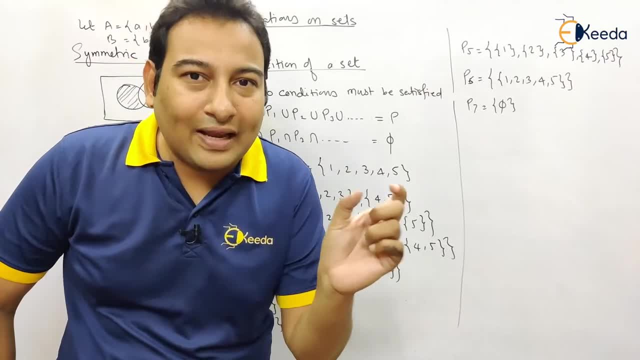 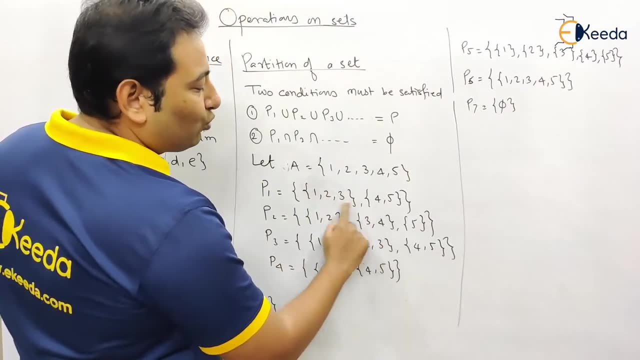 And the second condition is: if you take intersection of any two sets, we should get phi. Let us check what this exactly means. It's very simple. See here: If you take union of these two sets, you should get the original set. 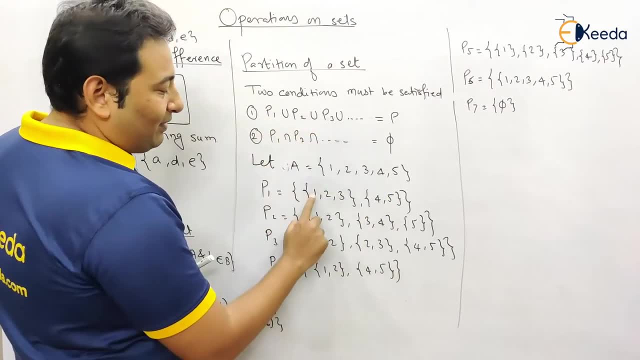 Are you getting or not? This is the first condition. P1,, P2,, P3 means this. So if you take union of these two sets- 1,, 2,, 3,, 4, 5, you are getting the original set. 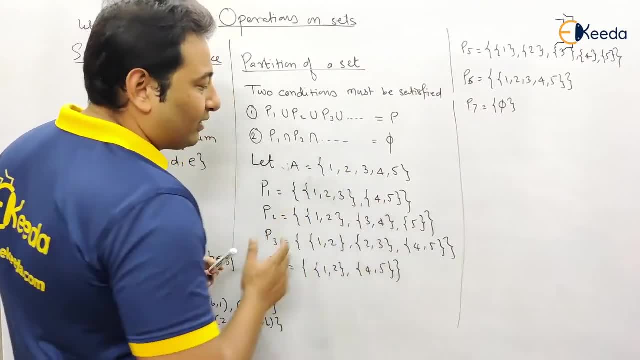 And the second condition is there should not be anything common between these two sets. And the second condition is there should not be anything common between these two sets And the second condition is there should not be anything common between these two sets. So if you take the union of these two, 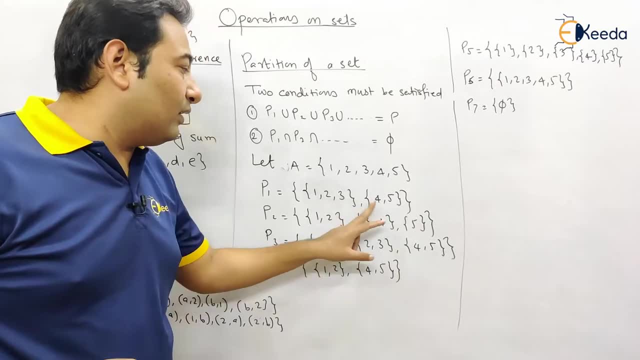 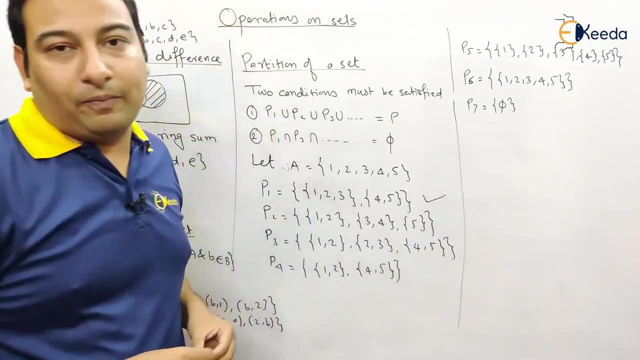 you will get 1,, 2,, 3,, 4,, 5.. And there is nothing common. If you take the intersection, there should not be anything common. So both the conditions are satisfied. It's a proper partition. 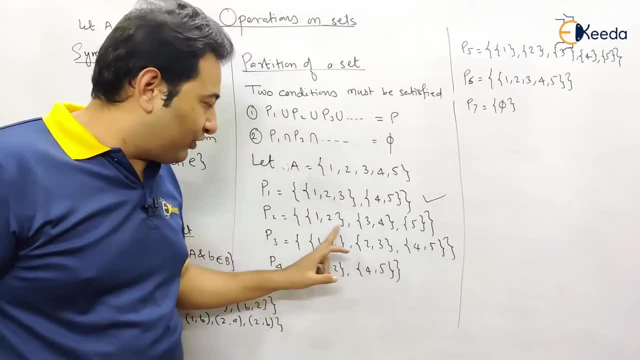 Let's discuss the next example, P2.. If you take union of these three sets- see here 1,, 2,, 3,, 4, 5, you will get the original set And there is nothing common between all the three sets. 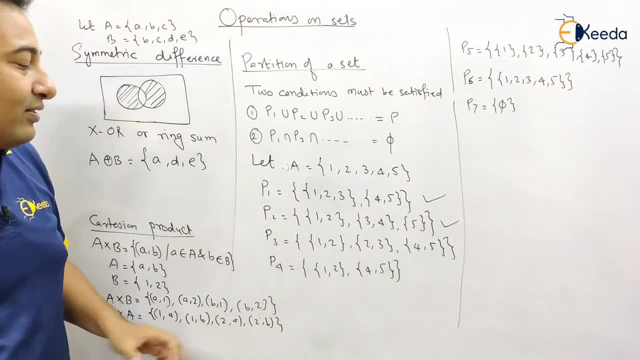 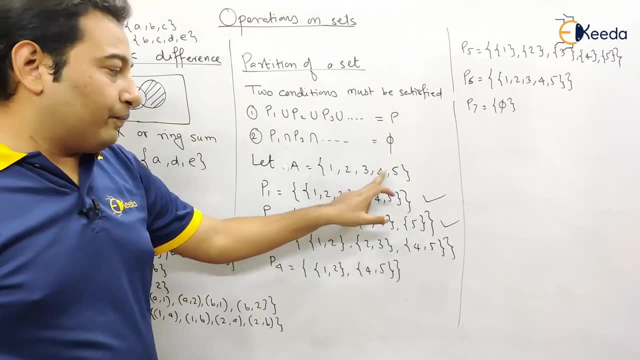 Therefore, it's a proper partition set. Let's move on And let's discuss the third case. If you take union of these three sets, You will get the original set A. You will get the original set A, But the problem is: 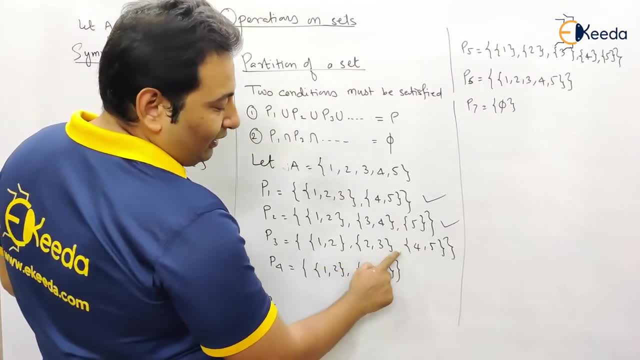 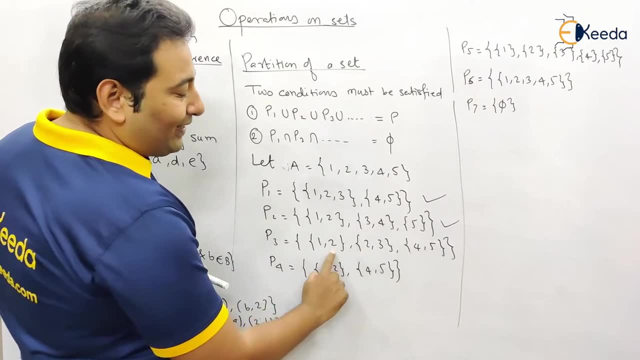 see here. all the elements are present. 1 is there, 2 is there, 3,, 4,, 5, all the elements are present. If we take union of these sets, we will get the original set. But the problem is if we take intersection of these two. 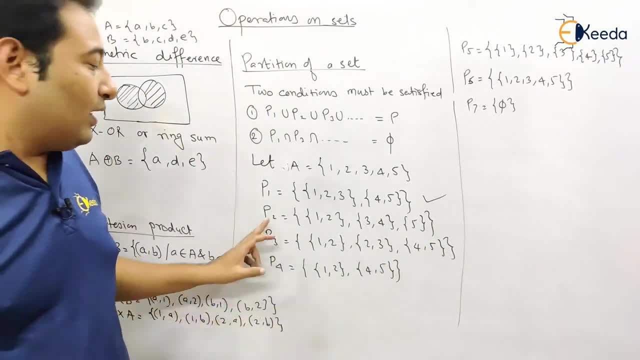 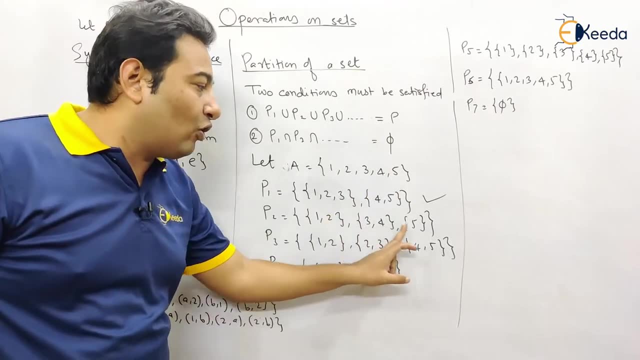 proper partition. let's discuss the next example, P2. if you take union of these three sets- see here, 1, 2, 3, 4, 5- you will get the original set and there is nothing common between all the three sets. therefore it's a proper partition. 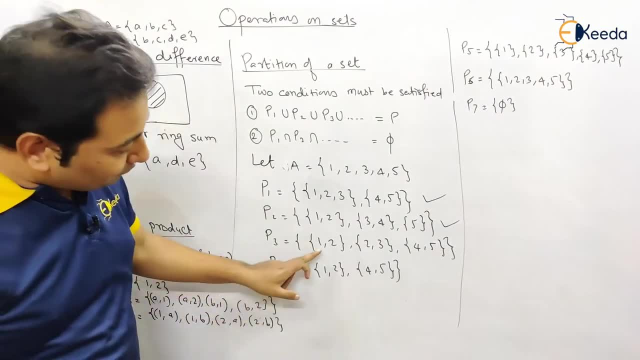 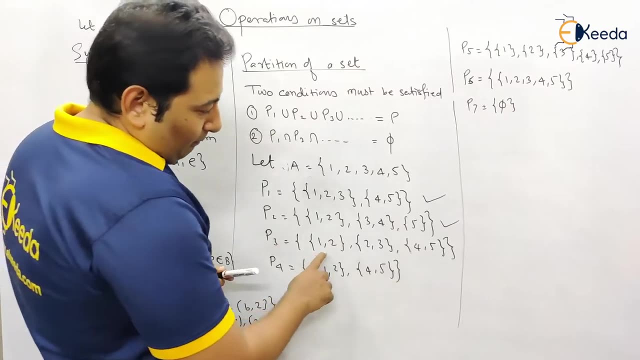 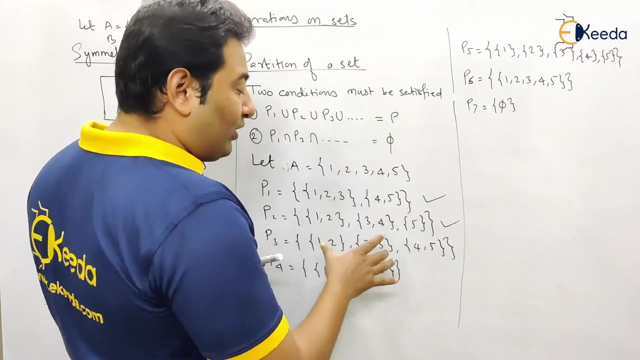 set. let's move on and let's discuss the third case. see here, if you take union of these three sets, you will get the original set A. but the problem is: see here, all the elements are present. one is there, two is there three, four, five. all the elements are present. if we take the union of this, 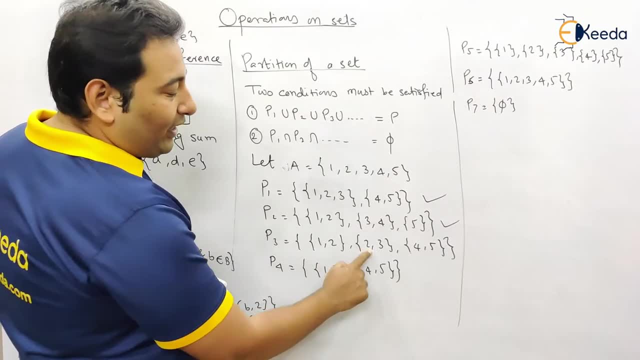 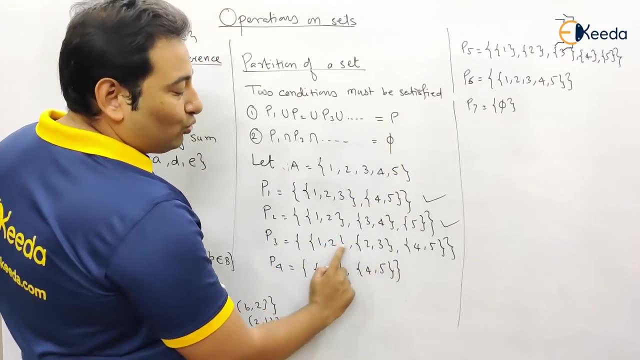 set will get the original set. but the problem is, if we take intersection of these two, intersection of all the sets should be null. if you take intersection of these two sets, there is a common element two. therefore, condition number one is getting satisfied, but condition number two is not getting satisfied. 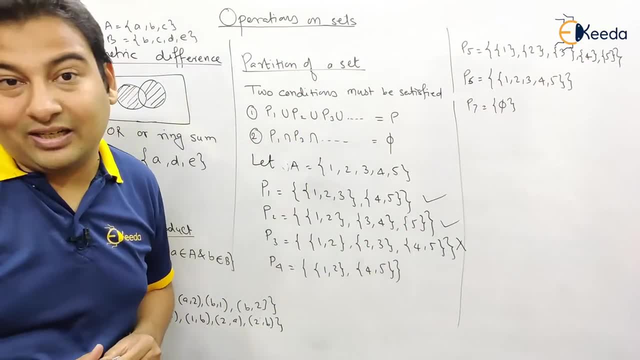 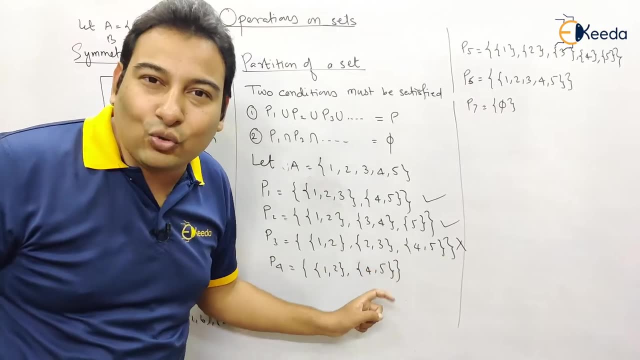 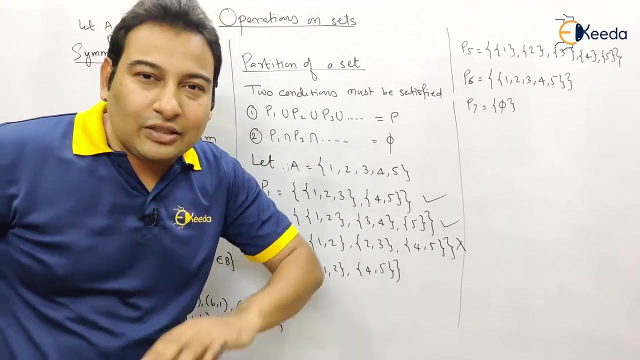 therefore it's not a proper partition. both the condition must be satisfied. is this clear? if you take union, you're getting the original set, but the problem is, if you take intersection of these two, you are not getting null. so there should not be anything common here. the common element is two condition. number two is not satisfied. therefore it's not a proper partition. 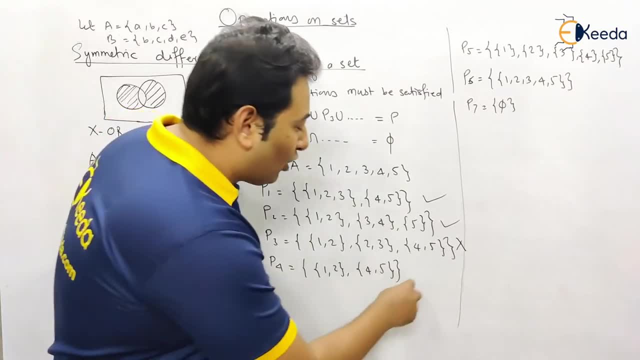 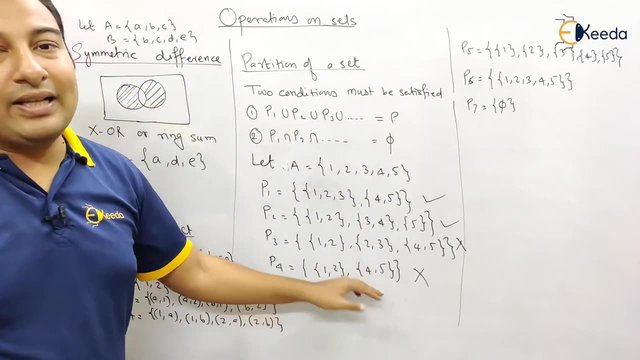 next question. let's discuss this. this is not a proper partition. why? because if you take union of this, you are not getting the original set. which term is missing? three is missing. therefore, it's not a proper partition. what about this? it's a proper partition why, if you take union of this? 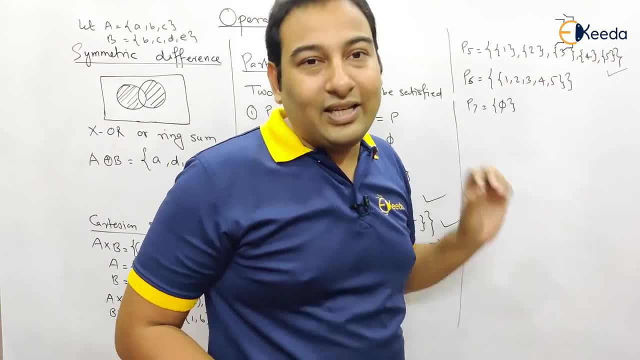 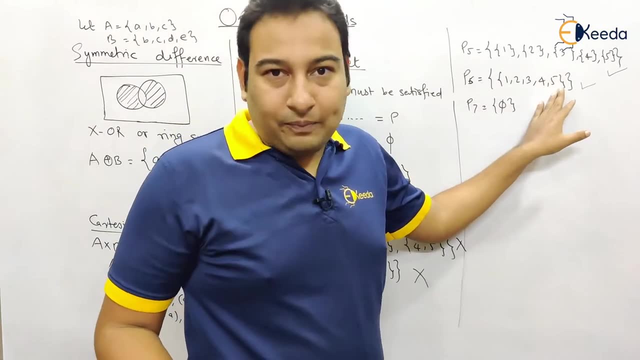 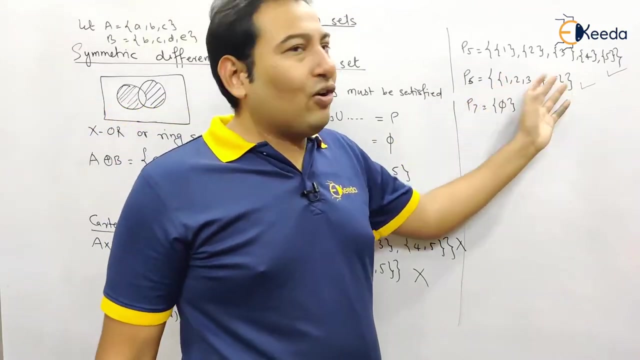 we are getting all the terms and there is nothing common between any two sets. therefore, it's a proper partition. what about this? it's also a proper partition because there is only one set. therefore, if you take the union, you will get one, two, three, four, five, and there is nothing. 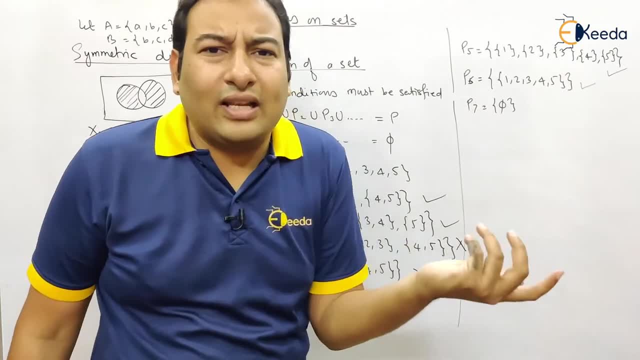 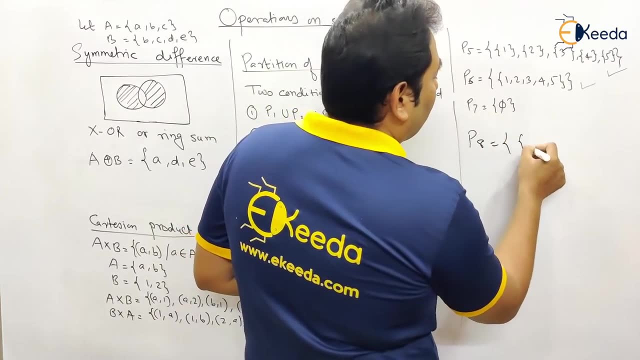 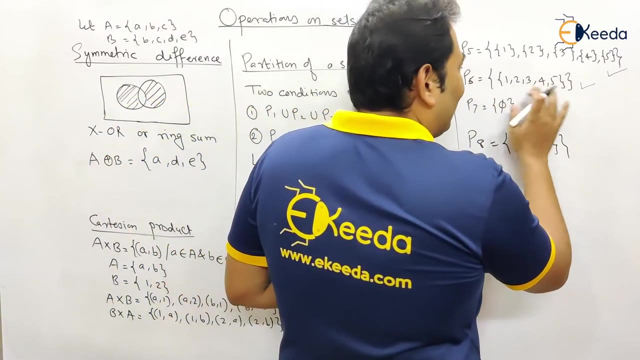 common between two sets? if there is only one set, so there is no nothing to check, and that one set should contain all the elements. suppose there is something like this: only one set. now it's not a proper partition because one- two is not equivalent to this. there is only one set containing all the 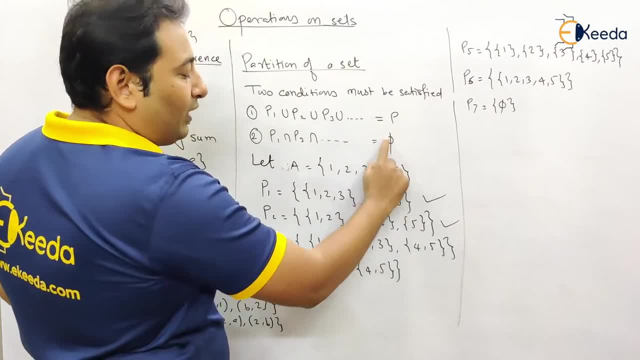 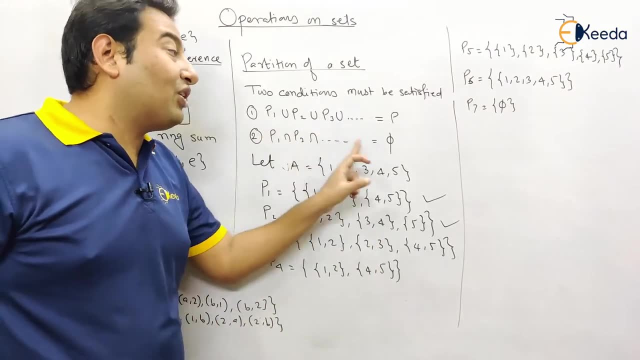 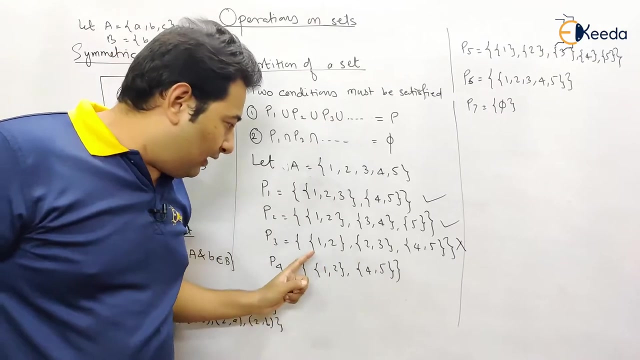 We will get the original set. Intersection of all the sets should be null. If you take intersection of these two sets, There is a common element 2.. Therefore, condition number one is getting satisfied, but condition number two is not getting satisfied. therefore it's not a proper partition. both the condition must be satisfied. is this clear? if you 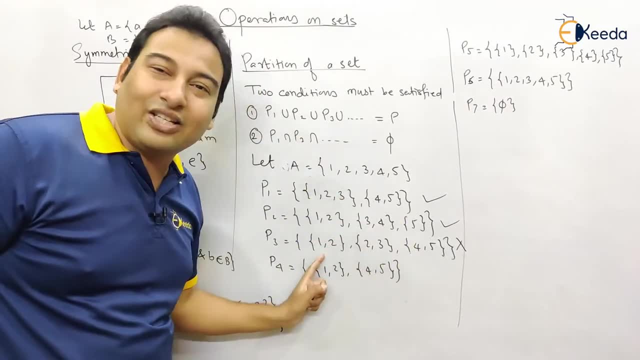 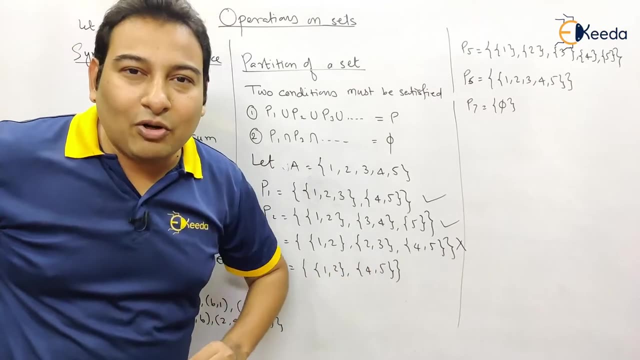 take union, you're getting the original set. but the problem is, if you take intersection of these two, you are not getting null. so there should not be anything common here. the common element is two. condition number two is not satisfied. therefore it's not a proper partition. next question: 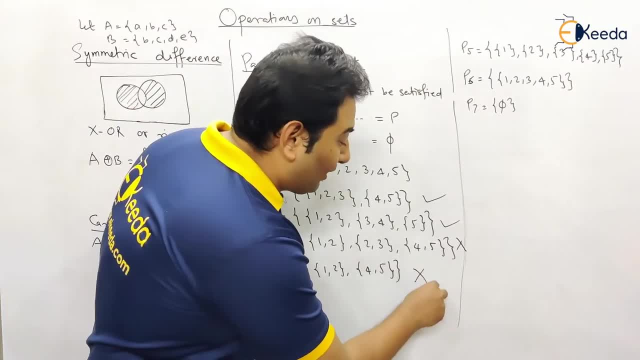 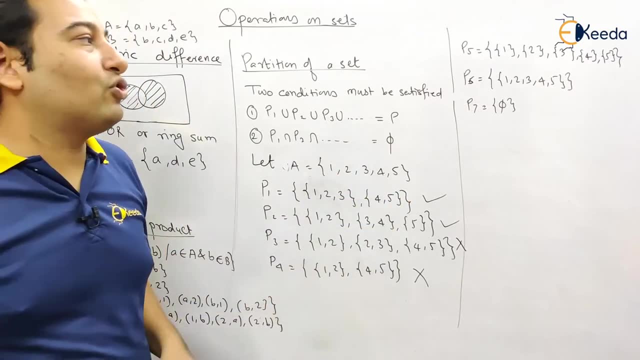 let's discuss this. this is not a proper partition. why? because if you take union of this, you are not getting the original set. which term is missing? 3 is missing. therefore, it's not a proper partition. what about this? it's a proper partition? why, if we take union of this, we are getting all the terms. 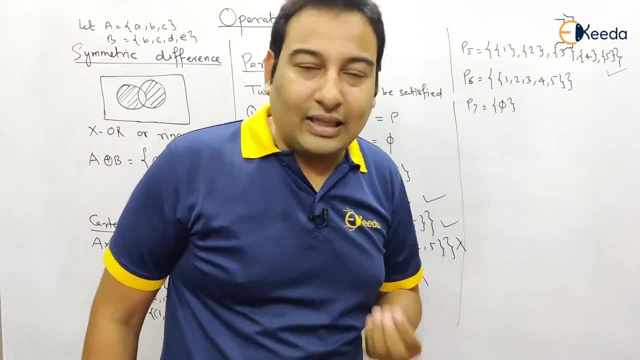 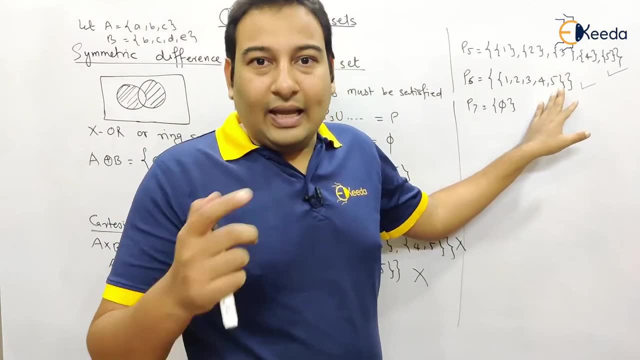 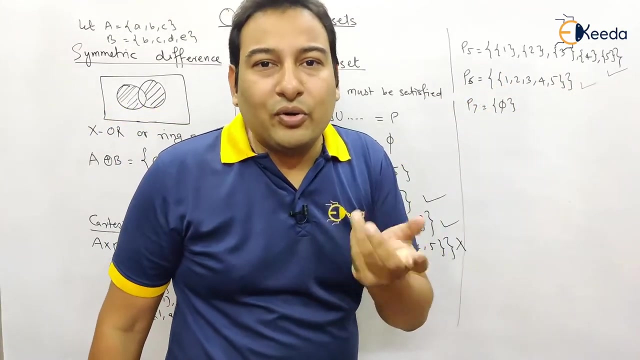 and there is nothing common between any two sets. therefore, it's a proper partition. what about this? it's also a proper partition because there is only one set. therefore, if you take the union, you will get one, two, three, four, five, and there is nothing common between two sets if there is. 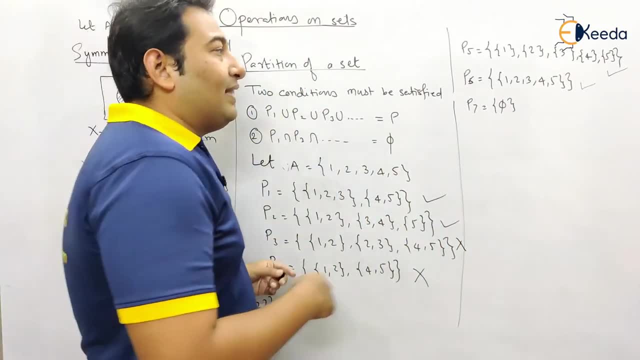 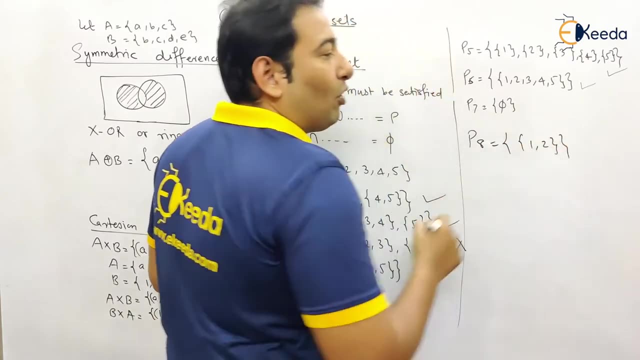 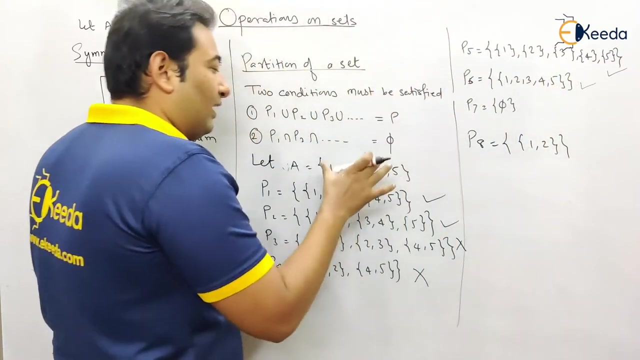 only one set, so there is no nothing to check, and that one set should contains all the elements. suppose there is something like this: only one set. now it's not a proper partition, because one, two is not equivalent to this. there is only one set containing all the elements. therefore, 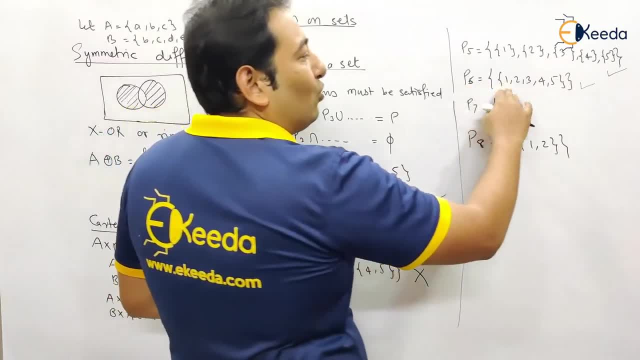 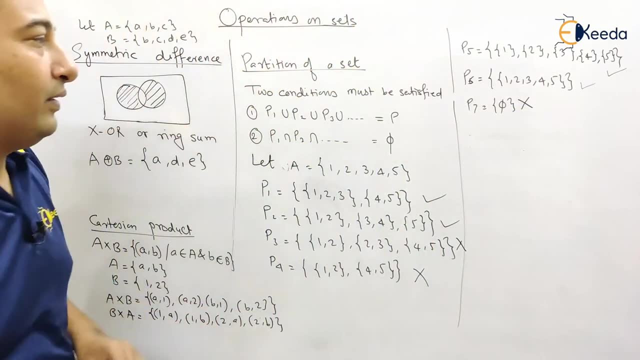 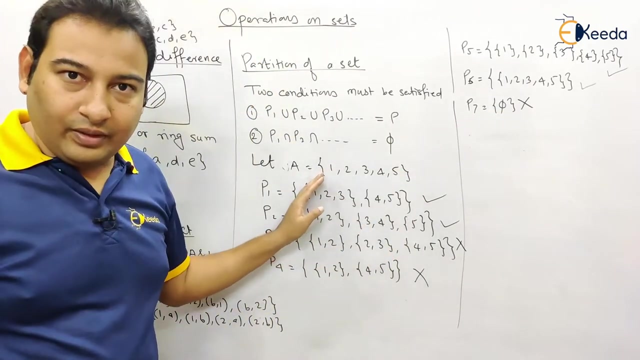 we getting the original element and no, there is no other set to compare. so this is a proper partition. and what about this? this is not a proper partition. is this clear? because there is nothing in the set and if you take the union, you should get the original set. so if you don't, 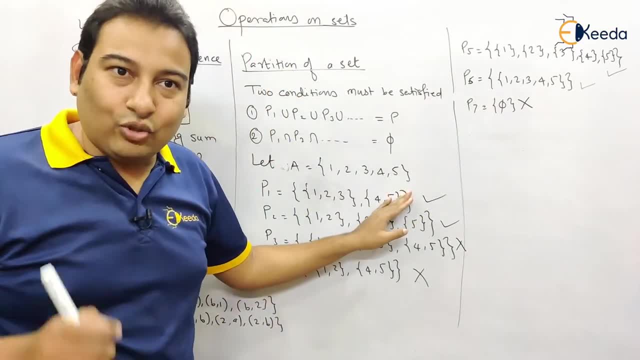 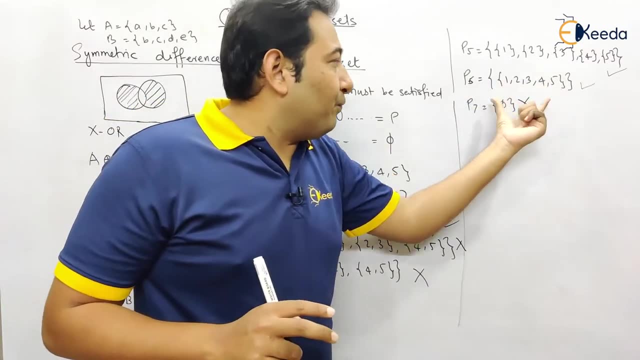 have anything. how can you get the original set? so the condition is: from this, you should get the original set. and the second condition is: there should not be anything common here. there is nothing. so how can you get the original set? so there is nothing in the set. therefore it's not. 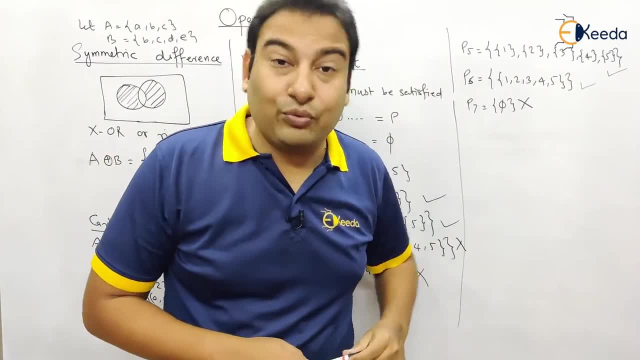 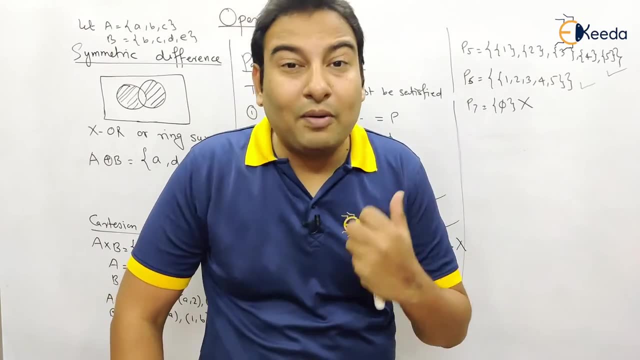 a proper partition. are you clear with the concept of partition? it's very important. so that's it. we're done with all. the operations started with union, then we discussed intersection, then we discussed complement, power set, semantic difference and cartesian product and finally we discussed partition of a set. so these